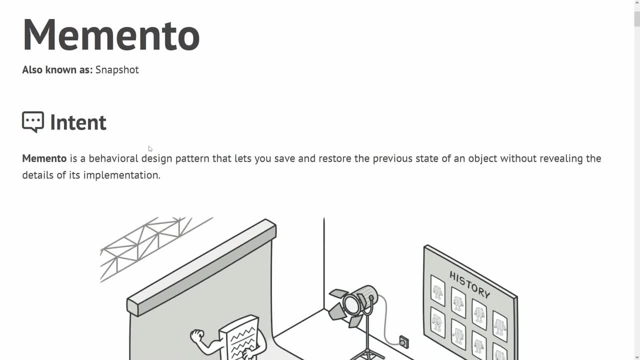 jeez, should have went into privacy mode. I'm messing around. Anyway, appreciate you guys for tuning in. If you enjoy this video or you're going to leave, don't forget to hit like first. That means a lot, Helps a lot to support And leave a comment with whatever you want. 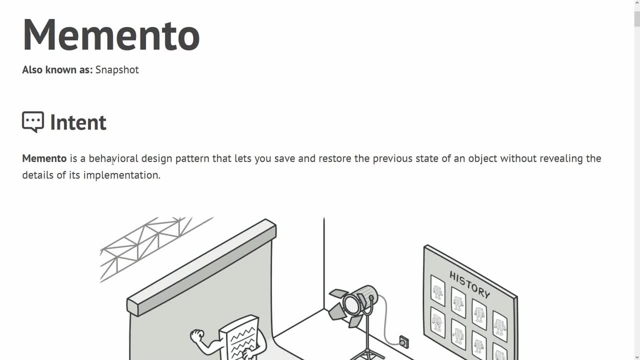 I'll try to answer all of them within the first few days And, yeah, let's just talk about memento and a little bit about expectations for this video. Essentially, I'm going to be coding it up in C++ And I'm going to start with the example from this website, but we're going to 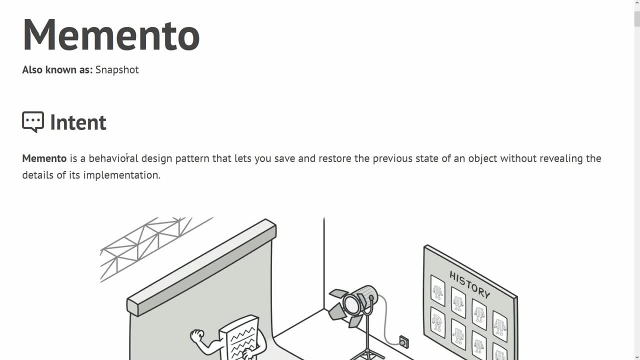 modify it a lot and talk about a lot of different angles. So essentially, the conclusion I came on this: there's approximately four different, pretty well-known ways of doing this And in this example they show one Which is probably the best in my opinion, But it doesn't mean you shouldn't know about the others. 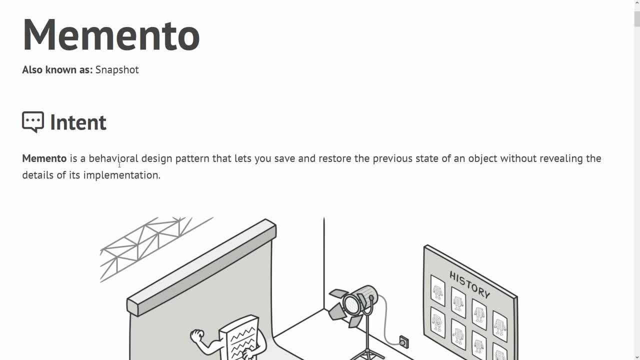 because the others? well, as you'll see, some languages lack the support to do this main method, So you might have to use one of the other methods of implementing the memento if you're not using C++ or something. I think it's mainly like PHP. I don't know all the languages. man, All right, PHP. 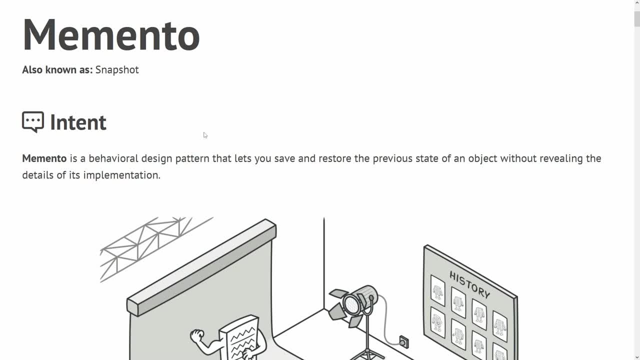 doesn't have this method, notably. but we're going to stick with C++ anyway. That's what we tend to do on this channel, in case you're not familiar with it. Anyway, we're going to stick with this way anyway. That's what we tend to do on this channel, in case you're not familiar with this. 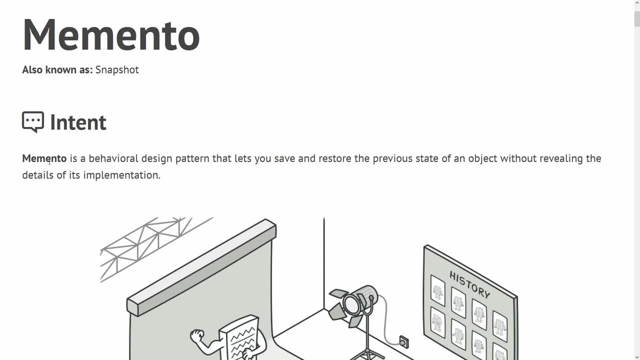 In case you're not familiar with this, we're going to stick with C++ And I'll see you guys in the next video. you're not familiar with that? Yeah, let's, let's go. Memento is a behavioral design pattern. lets you save and restore the previous state of an object without revealing the details of its. 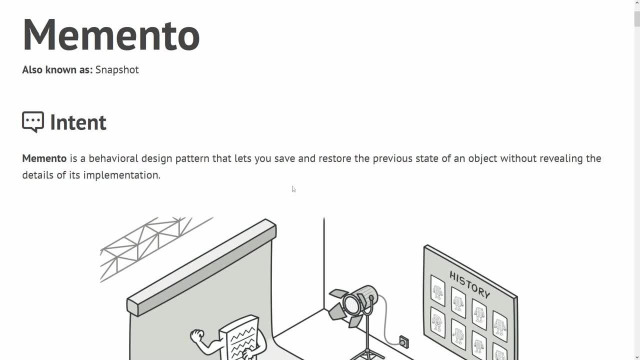 implementation. So it's sort of like the undo button. You can also use it as saves sometimes, or a version of it for saves, Yeah, so let's dive in a little bit more. I'm not going to talk too much. We're going to dive into the code very shortly here, but I'm going to at least try to. 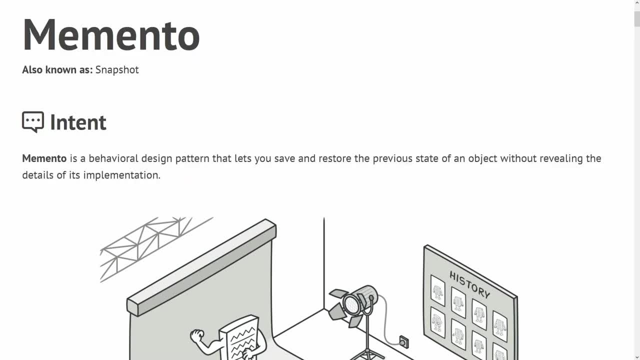 hit the main points, like the overview, or what it essentially does. So you know, it saves a state and it restores a state, but it does it without revealing the details. Okay, we'll get into that Now. you all know it's pretty simple to just make a copy of a struct or something along those lines. 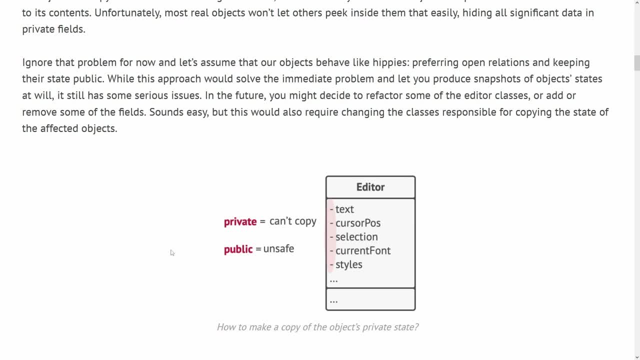 or copy a bunch of variables and then restore them. You should know how to do that. if you're a coder in any sense You know. if you know how to make another variable of the same type and assign it something from one that's already instantiated, You know that's a copy. So 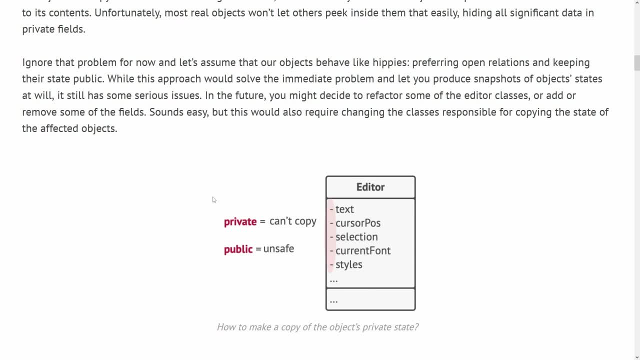 this. you know this is something you can just hack together and put in there and chances are you have. But with this pattern it makes it very maintainable and very easy to expand, Very easy to add to basically any class. And there are some drawbacks, We'll get into them. But yeah, the 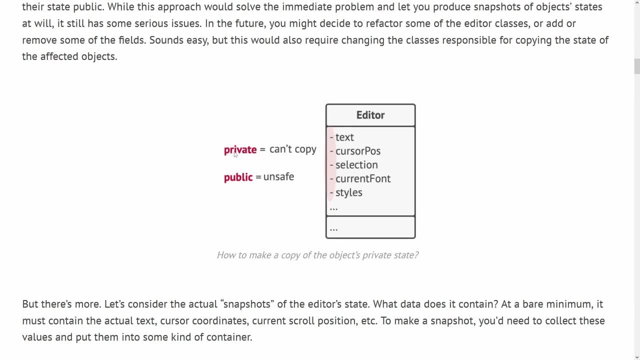 standard problem with classes is you have all your member variables as private, which means, well, here they say can't copy. What they really mean is can't access. So something trying to save wouldn't be able to access all those private variables, So you can't access all those private. 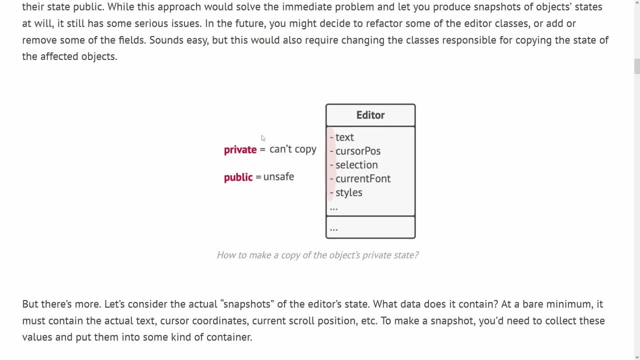 variables. You could make a bunch of getters and setters, But is that really how you want to design? Well, that's up to you, But generally this doesn't use a bunch of getters and setters. So that's nice, because it's not going to be that giant chunk of repetitive code, And that's essentially what you. 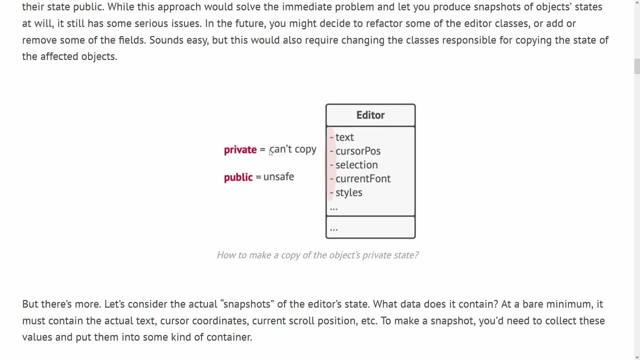 would have to do to get around, like the private problem here with can't copy. So we don't want to do that. That's just too clunky for what we want to do. So memento is going to be better. And they say, hey, your public data is unsafe. Well, we might get into this later. But for one of these, 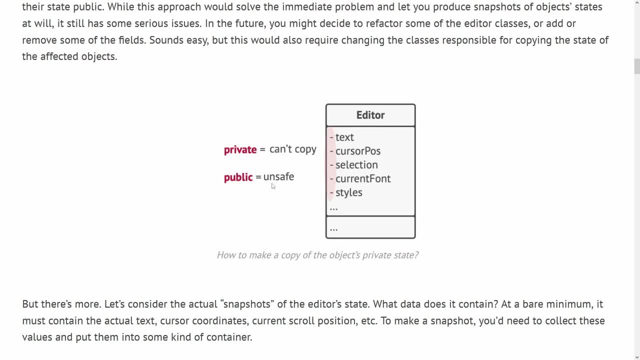 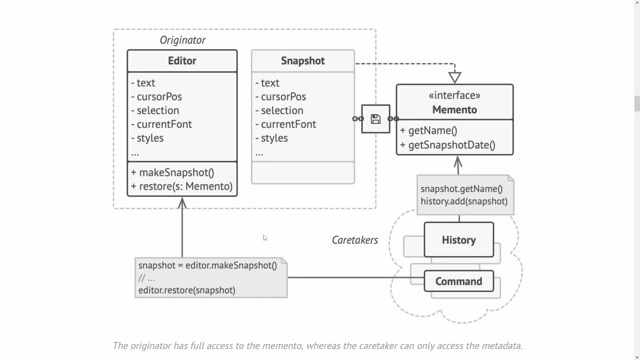 methods, you have to make it public, But for the others you can keep it private. So how to make copies of the object's private state Question mark, question mark. That's essentially what we're going to solve. Here's the little diagram of their example. Now keep in mind, with these examples, if 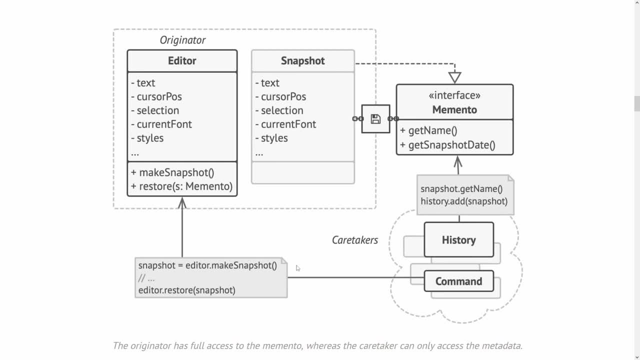 you're anything like me, you can study this graph all day and still have no flipping clue what it actually means. You know, and I know you can really dig in and understand it, But for me personally I kind of had to see the code. So we'll get to that soon. But this is supposed to be a diagram of how. 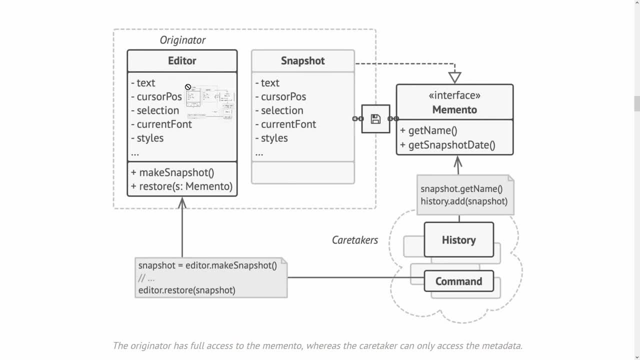 it works Now. essentially, you have what they're calling an originator, Which is over here, And that is basically what you're working with. That's what you might want to take snapshots of, And you can see they've put methods here for make snapshot and restore. And restore takes a memento, That's. 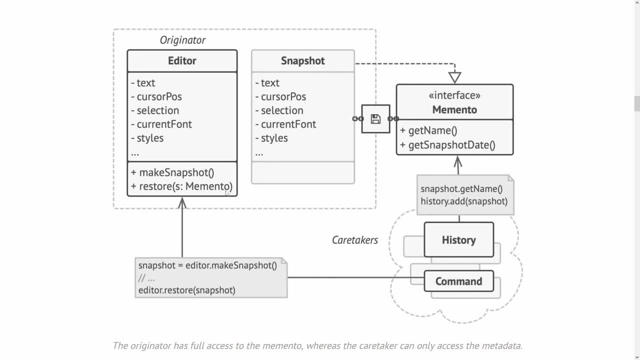 what they're calling it. You don't necessarily have to call these snapshot and memento. You could just call it like whatever We'll. We're going to stick with this, though, But I always- I say this a lot in all my videos, because 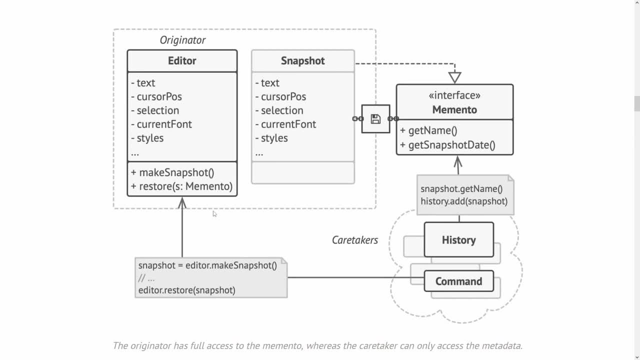 people really get hung up on variable names- I know I do And like these words in these boxes. they don't matter, They could be a, b, c, d and you know some functions, But it helps to uh for them to make some sort of sense. So they're talking about the context of a text editor with these. 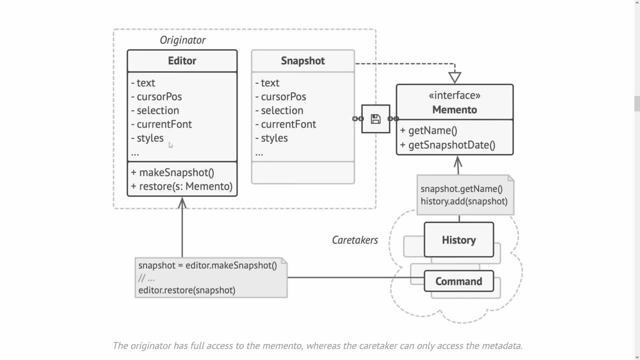 examples. That's why you see text cursor, pause, selection, current file, whatever It could. These could be anything, though They could be positions. If you're saving the state of a 3d object or something like that. Like 3d positions, You could have a lot of different. 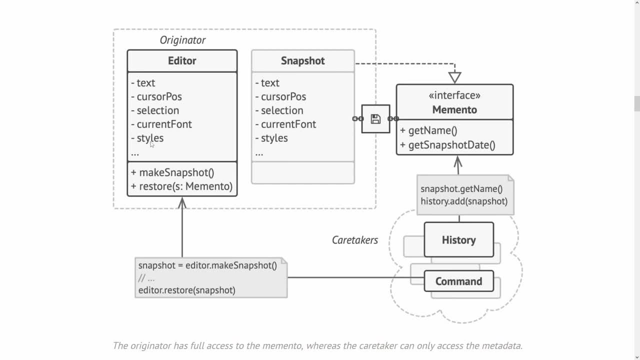 stuff. But for sake of example, you could think of these as a, b, c, d, e, because who knows what they really are, you know, Anyway. so we got make a snapshot and restore. So what's a snapshot Now? the snapshot has all these same member variables as this editor- Basically everything you'd want. 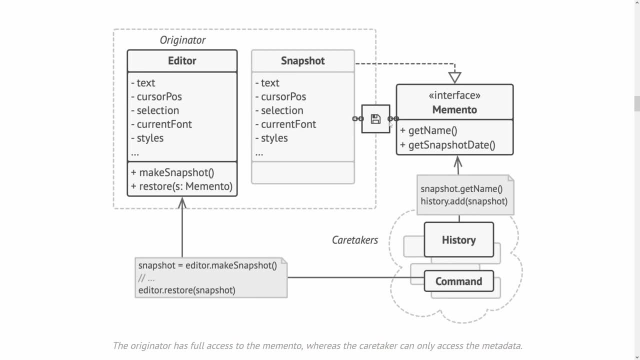 to potentially save. So they have a little save button with chains. Who knows what that means? They've got a dotted arrow with a triangle. Who knows what that means? Something about interface, Something about save operation. That's why I don't understand these charts. It's never clear what all these mean. So 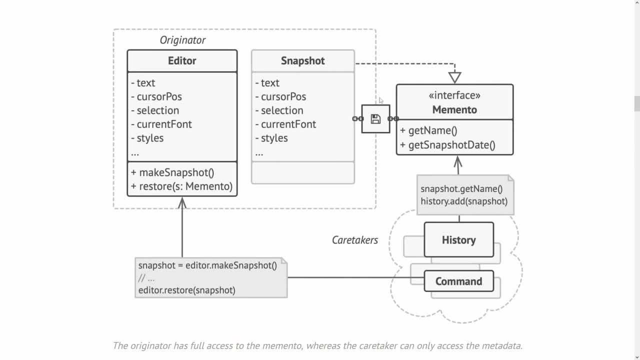 I don't know Well, why is this in a dotted line box? Who knows? But I think what they're trying to allude to with this graph- And it's not their fault that I don't understand the graphs. Let me be clear. I think it's. it's purely a me thing. The point is, I don't think it's going to work. 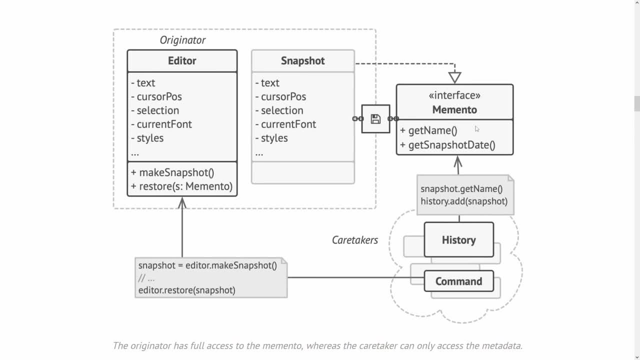 for everybody. If it doesn't work for me, it probably doesn't work for a lot of people. So I think it's just me. That's all I know. They have a lot of stuff to do with this, But here's the point. Here's the point. 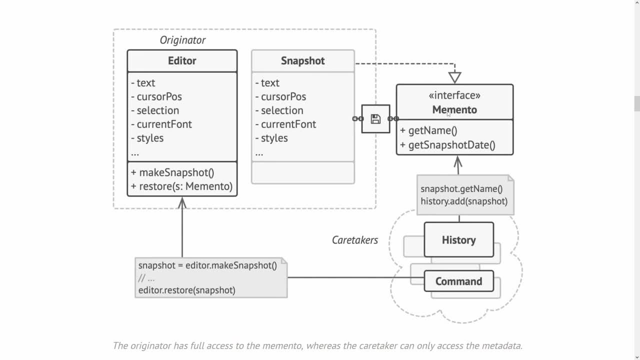 Out of data. we actually have data, So you can go back to the memory interface. Let me talk about that a little bit And we can kind of try to see. So what we want to do is we want to go back to the memory interface And we want to go over here, Interface Memento, All right, And in this, 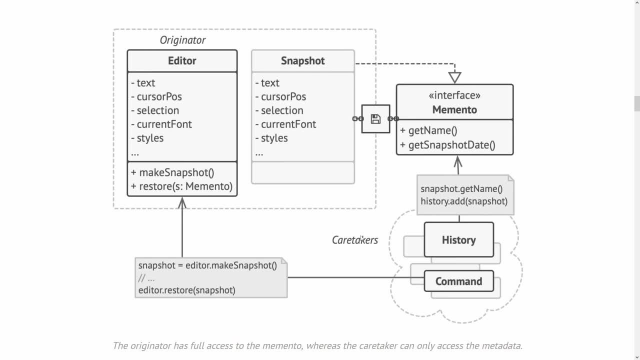 interface. they have a git name and snapshot data, So we kind of have to unpack what this is: Some memento interface that has git name and it has git snapshot. Oh, it's date, Git, snapshot, date, All system and a caretaker. you could probably call this caretaker something like a mediator. it might. 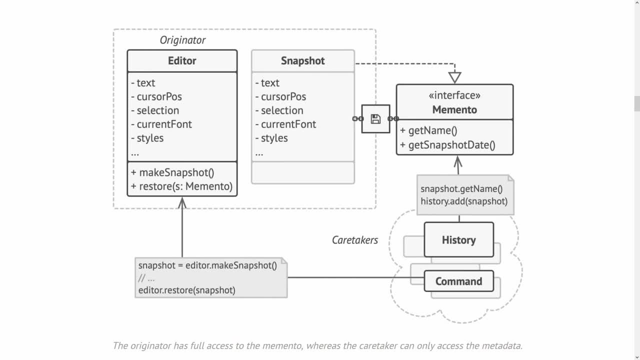 follow a pattern pretty close to that actually, if you want to look up mediator at some point. but essentially what a mediator or caretaker does is it helps handle the interface between two objects and in this case it's this memento interface that handles editor and snapshot by calling these: 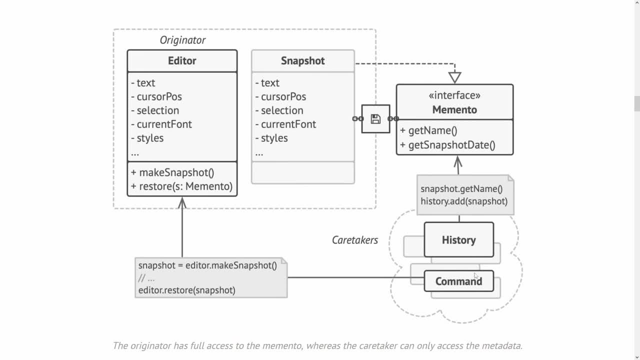 functions and it also, i believe, the caretakers where you're going to hold all these snapshots. so it's going to be the one that's doing this whole restore and passing in info and grabbing the make snapshot data using specifically this memento interface. confused, yet good. good, me too. 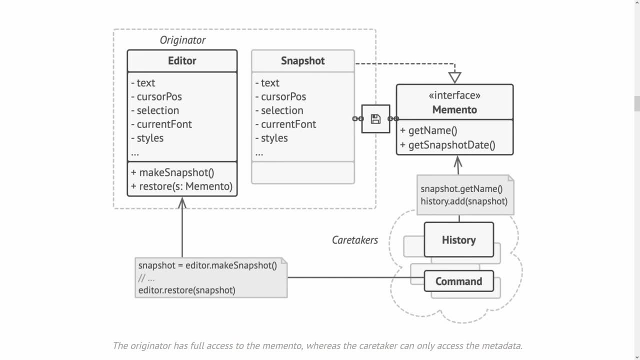 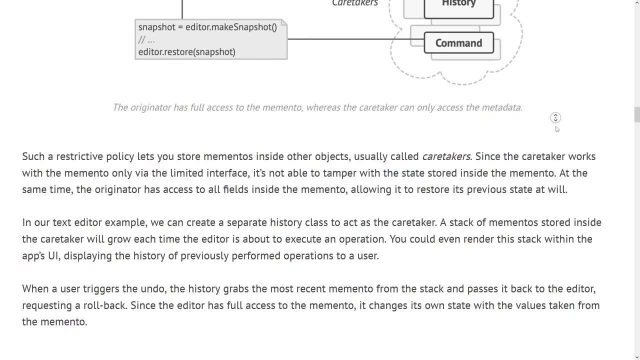 let's get to the example. and it'll make a lot more sense after that, or at least it does for me and kind of goes without saying. but you know, i gave you the link to this web page. if you really want to read all this stuff and dig in a little more, you can go visit the web page. 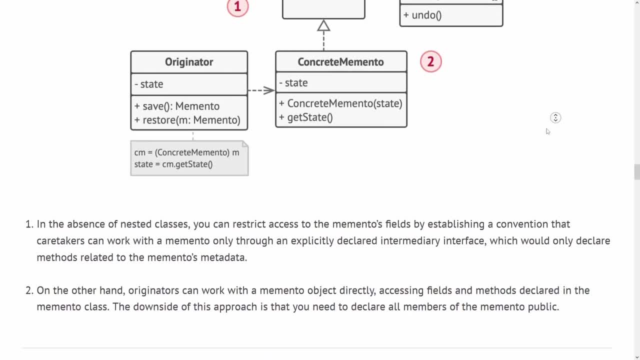 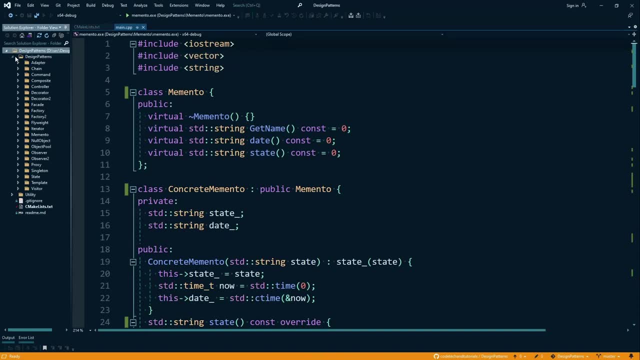 no one's stopping you. i'll even leave a link down below, but i'm going to kind of skip a lot of this and we're going to get into the code now. okay, here we go. we're in our design patterns repo. link to that down below. it's basically where i'm just putting all this. 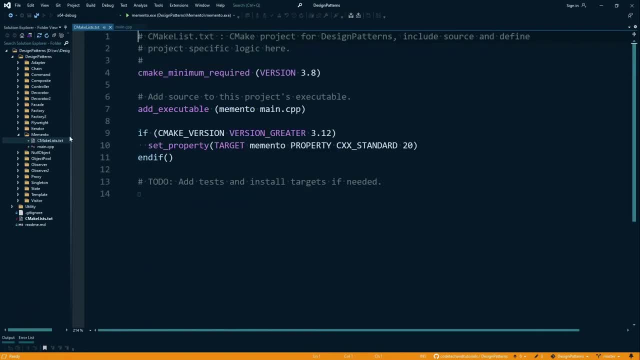 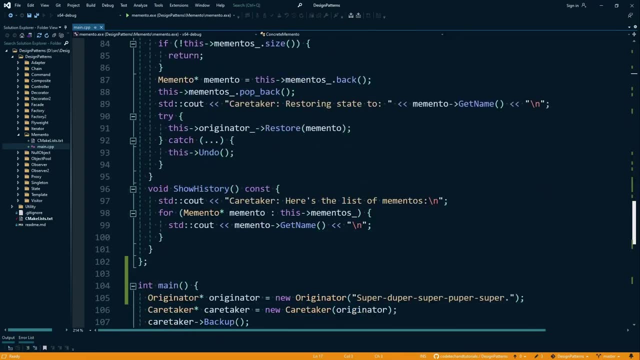 code and i've made a new folder here called memento. already got the cmake done and we just have a main. so the main has all the memento code up above just already ready to go. then down at the bottom i've got a main to test everything out. so we're not separating out into a new file, okay. 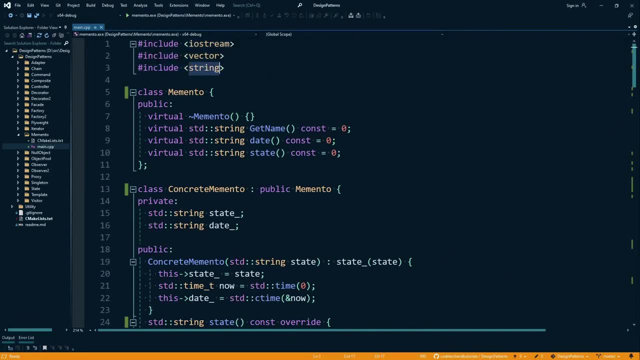 so we've got some pretty standard includes here: io stream vector string. we'll be using those. let's just go from top to bottom here and i will explain all this stuff. so we have our memento class now. notably, this is an interface we can tell because, well, the virtual 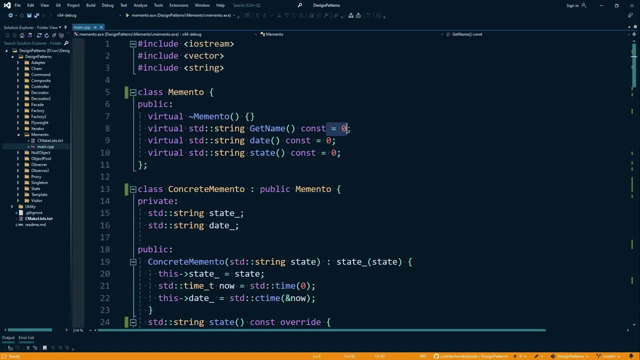 keywords, the virtual destructor, and mainly this equals zero, means there's no definition. so if you inherit from this class, you inherit from this interface. you have to make these methods, you have to make your own version of these methods. that's just part of interfacing in c plus plus and this uh whole equal zero thing. so uh, let's go to. 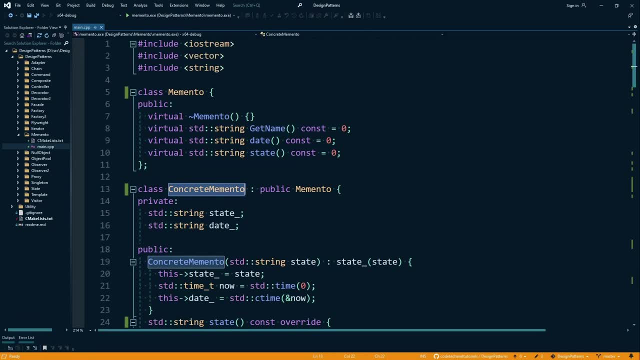 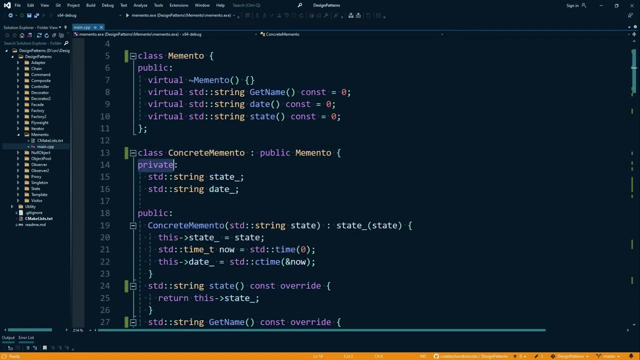 the next one. so next they have a con, what they call concrete memento, and obviously it inherits memento, so we've got to make our version of these functions for that. but they also add a few things here in this memento they add a state and a date. those are private so nobody can access them. so 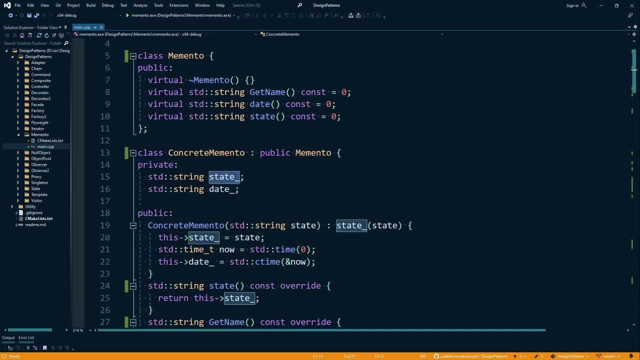 we're keeping track of state, and now you can see here, in the case of this example, this is pulled from that web page as our starting example: their data or their state. what they're calling state here is basically the state of the object or the save. it's just a string. now, in your world, this is 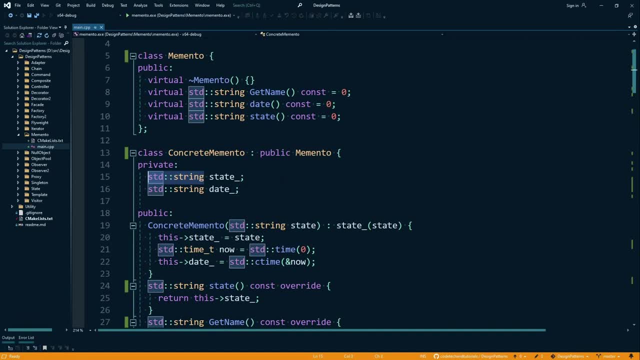 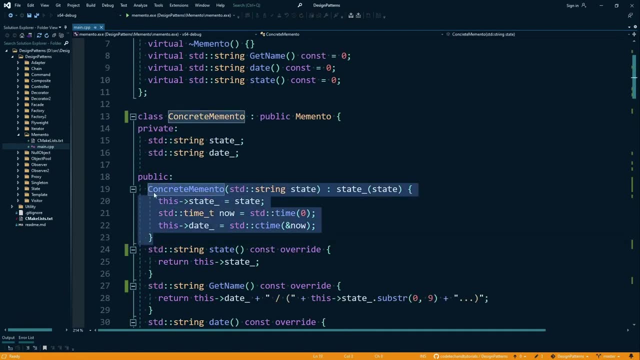 probably going to be some other struct or class that has all the info. but we're going to. we can. we can work with that a little more later if we want to play around, we'll play around at the end. so you can see they have a constructor, a little public constructor and the constructor. 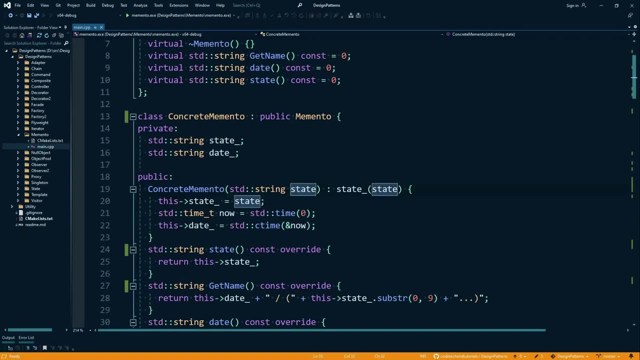 takes a state. you've got to construct this memento with a state. that's really important, because you can't just create one with no state. it's got to have something already there, so you can't really just create these easily. you've got to have something ready to go and, as you can see, it just sets the state and the strings. in this case, 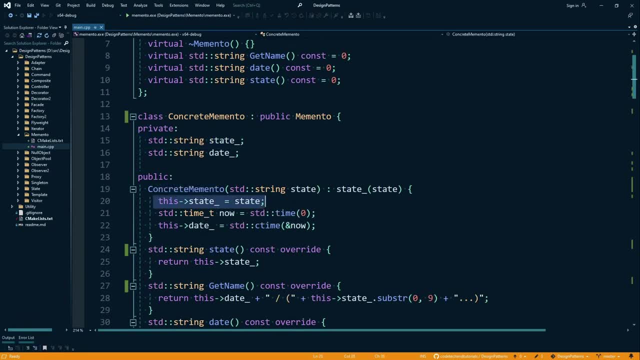 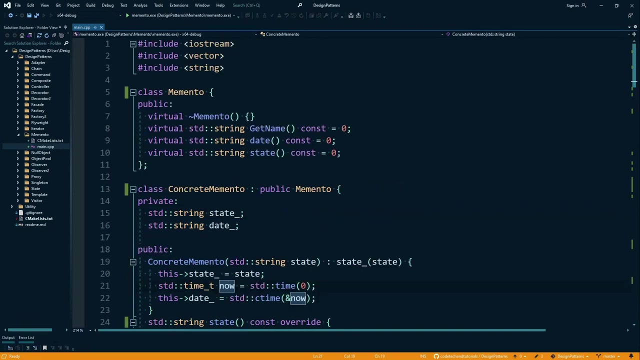 but consider it could be any object. so there we once again set the state. not entirely sure why they do that twice might just be a bit of oversight on their end, kind of odd, but that's really important to keep in mind if you want to trying to cut down on this thing, or it's pretty. 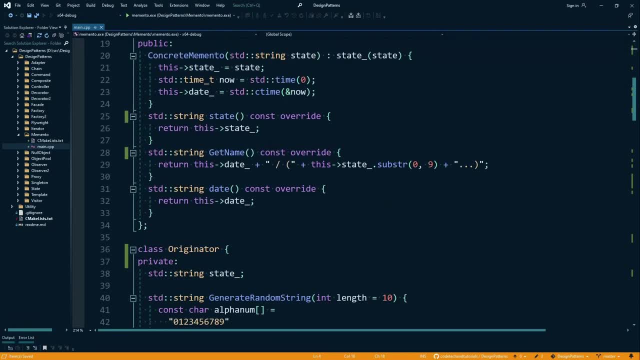 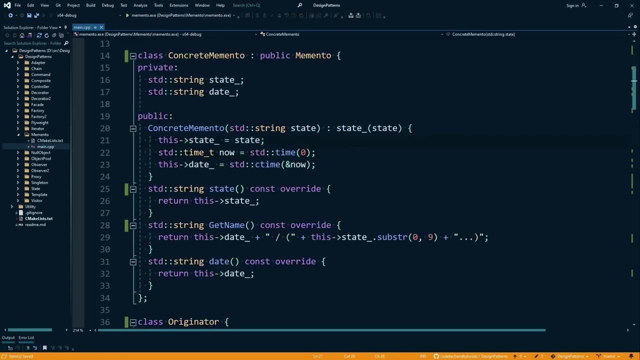 maybe, if you know, it's going to be your identifier again, we'll just keep it as it is and i'm going to drag this up and we'll see what it looks like. it looks like to me. this is just one of those things. that's something that i'm going to check somewhere and then we'll see what's coming out of. 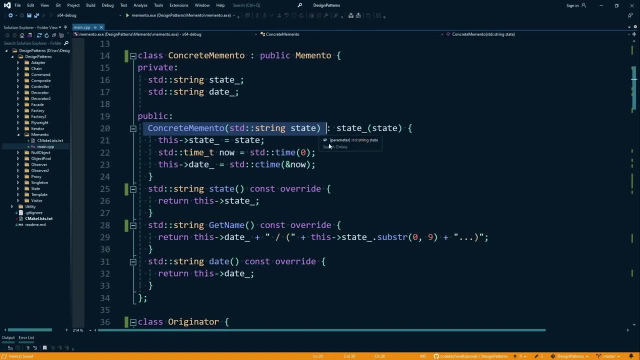 there eventually going to create a timestamp of when you created it, which is a fine feature to have. you might as well. so that's why they got this string date here, to keep that. and the way they obtain it is they make a time t variable called now and set it to time zero. that's just part of the standard library. 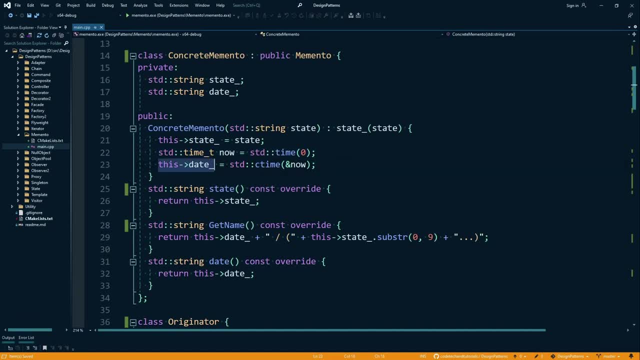 there so you can look those up if you need more info. and they set the date to the c time now. now, what c time does is, if you pass it one of these times is it returns a, a care pointer, which is essentially a string. so that's why they're saving it to the string. c time is returning the time as. 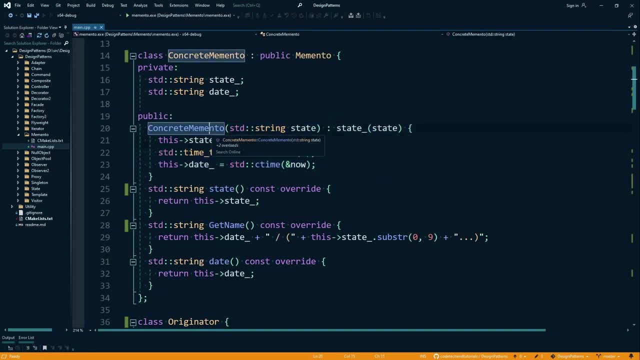 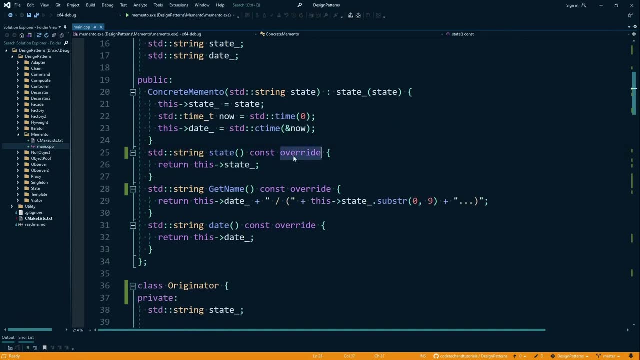 essentially a string. all right, so cool. create a memento with a state and it's automatically going to make a timestamp. cool. what else do we need? well, we got to implement these functions and you can see there's a state here overridden. all it does is return the state, which needs to be the object type. 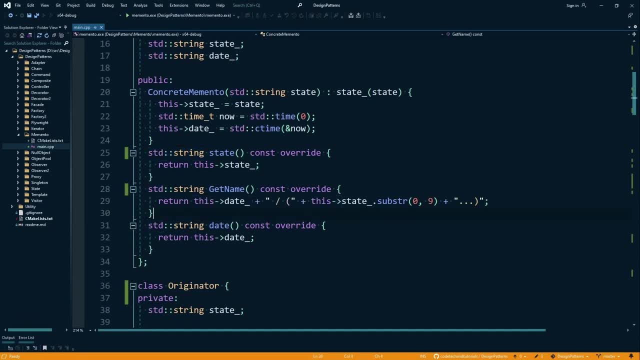 string here. so that's fine and we have a get name and you can see what get name does. it basically takes like returns, a string of starting with the date and some stuff about the state, so it's basically the name of the little save hash. in this case they're using a date plus the state's substring. 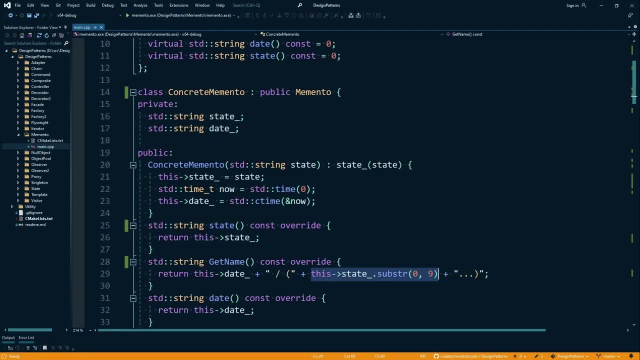 data up to up to eight characters or nine characters. so because their struct or their object for state is just a string. that's why you can do all this. you might do it a different way, like you might use the date, sure, but you might not be able to do this if you're only holding, like integers and floats and stuff. so you can get. 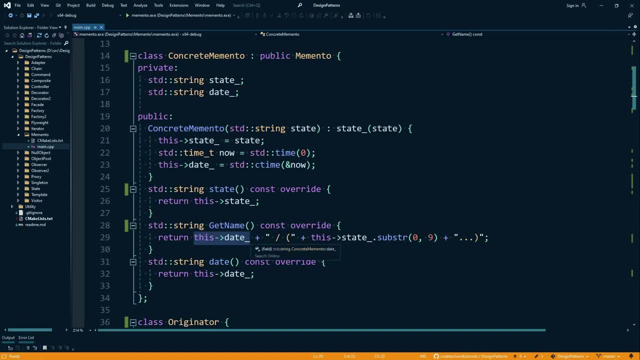 creative there and make cool names. they're at least all going to be different because the date timestamp is always going to be different as you create them, unless you can magically create two of them at the exact same time, which is going to be pretty hard to do. but i guess the point of me 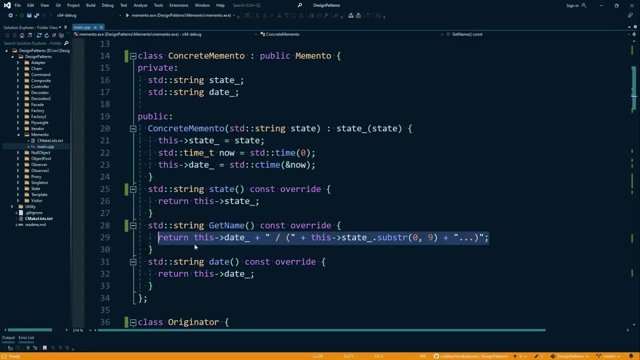 going on about this is to just let you know that you got to adapt. if things are going wonky for you, like if you happen to accidentally beating date stamps at the same time and object names of the exact same name, well, you're going to be able to create two of them at the exact same time if you're. 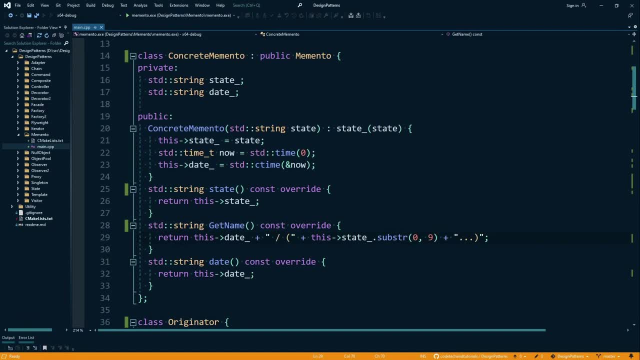 your names might overlap, and is that going to cause problems? i don't know. it depends. if they're in a stack anyway, with an undo button it might not matter too much. but if it does matter, you have to come up with some ideas to adapt. this is the point. 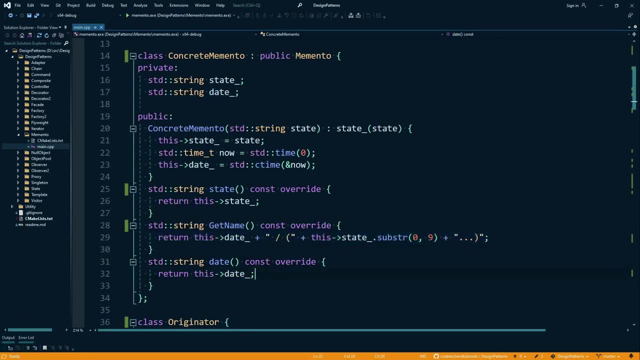 the date is just the date, just returns the date. so we've got all those implemented. we've got some private members for what we want to store. so that's essentially the whole memento right there. now let's check out the originator. this is something. this is what we're going to. 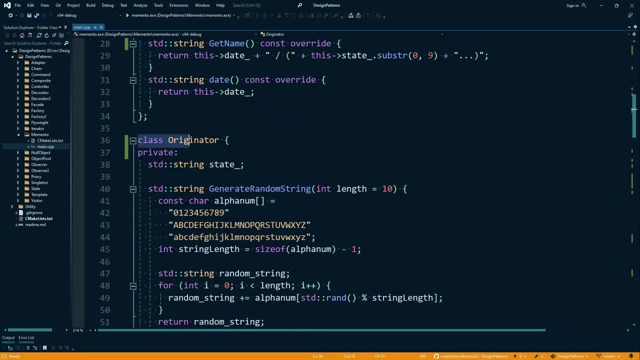 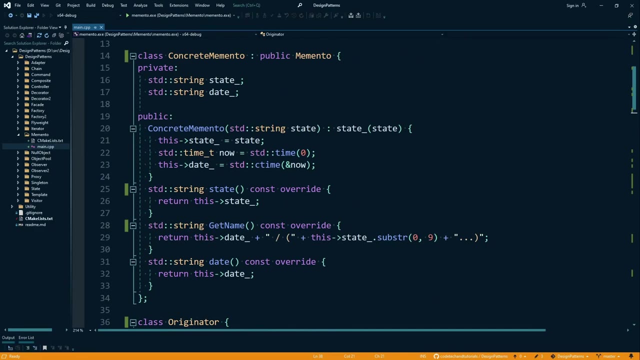 pull this state from essentially. so here it is. it's not inheriting from anything, so this could be any class, any class in your program that needs a save. essentially, well, you've got its state or its internal data, which is private. that's the main thing that needs to match up with your mementos and 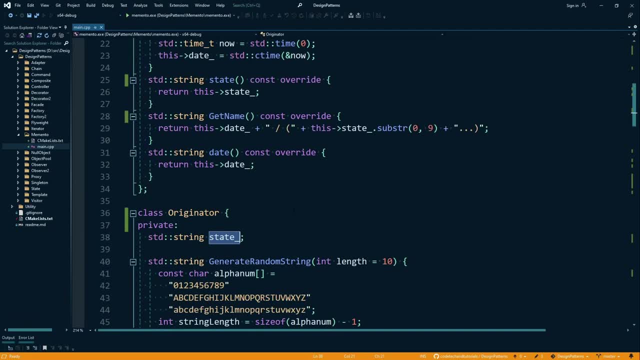 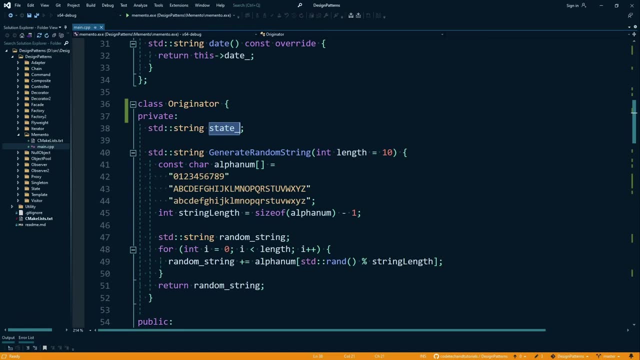 he needs to take all that private data that you would want to save and restore. now they've got some just kind of various code here that just generates a random string, which is kind of interesting because essentially you need some some differing data and they just made a little system to make. 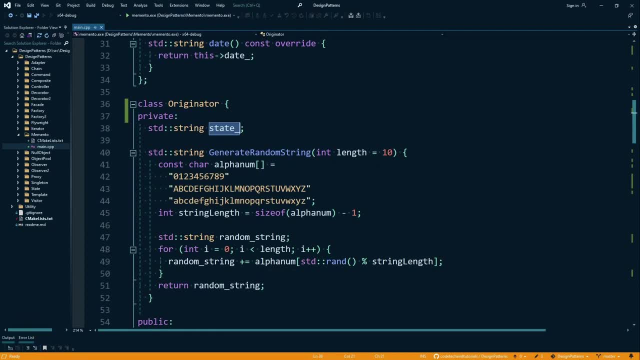 random strings and we can walk through it. i guess we would will briefly, but it's really not super critical, important uh to understand, to understand uh the whole memento thing. it's just their way of making random data. so they've got a const care of alpha numerical, just the. 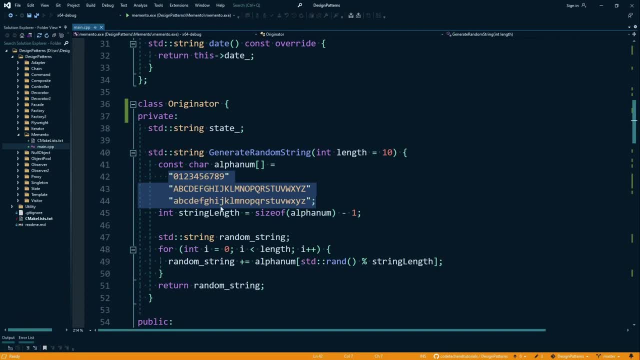 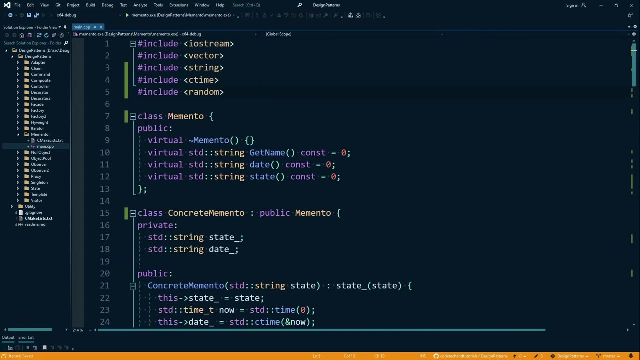 whole alphabet and, uh, all the numbers, upper and lower case, and they just get the length of this. and then, uh, they make a variable called random string and they use the rand front function, which we won't be able to use unless we include rand here. so let's do that. and they use the modulo. 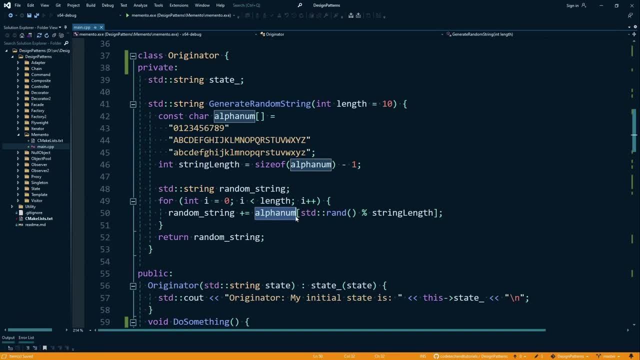 operator on the string length to go somewhere into this alpha numerical care array. so essentially they just do: a plus equals this is going to add to the string. so they just go for the entire length of whatever this thing was and uh, yeah, or this length comes from this input- generate length of 10.. so they just 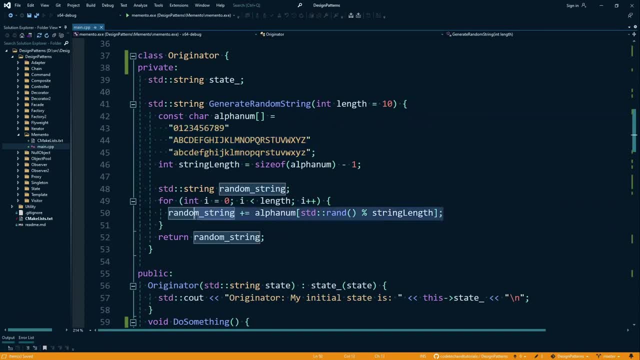 basically end up making a random string of all these characters. yeah, that's essentially what this is going to do, so i think we've walked through it enough. just, uh, you can see the brackets to index in there. it shouldn't crash, because this modulo should never be able to go. 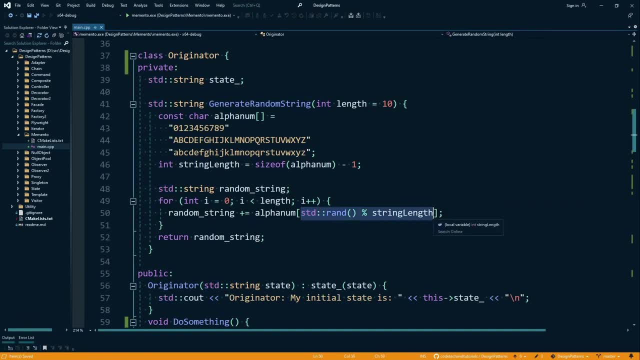 above string length. it's impossible. you don't know how the modulo operator works. it's a math function. definitely look it up if you don't know it, because you got to know it as a programmer. so i'm not going to over explain it anymore. i'll leave that to the math book stuff. but 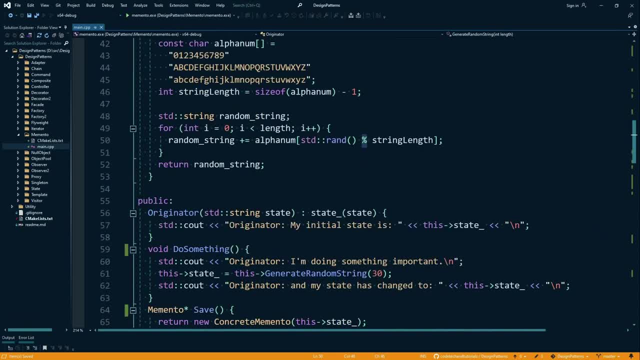 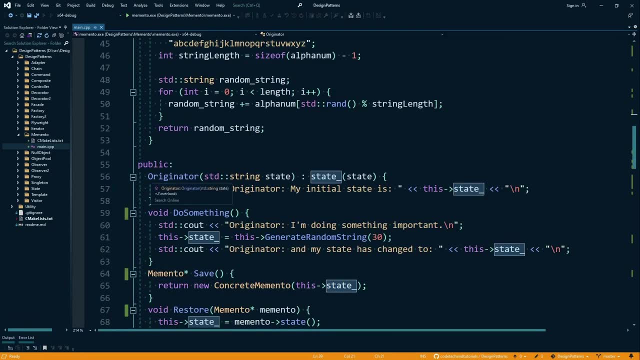 definitely look it up. you can look it up on c plus plus for reference. i usually tell you to all right, well, and then it returns the random string. so just some code to make a random state, basically. and then here's their public functions. uh, they started out with the state. if you want, 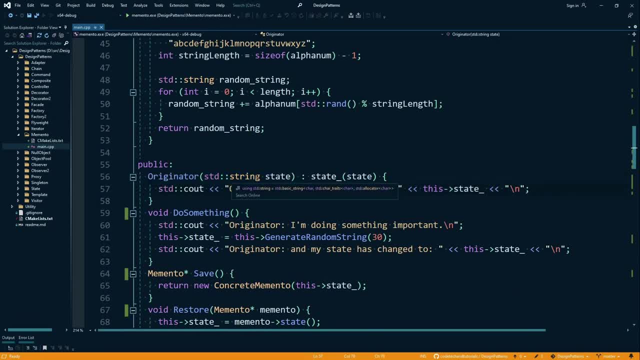 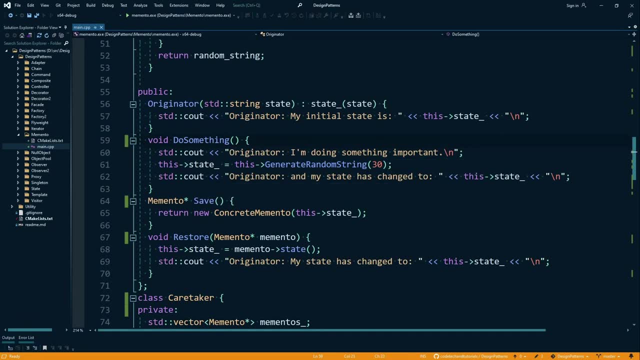 so they got originator that takes the state: uh, just a string, they've got some work. so of course your class is going to do something. essentially well it should. they've just got some generate random strings. so essentially when you call do something, they just change the. 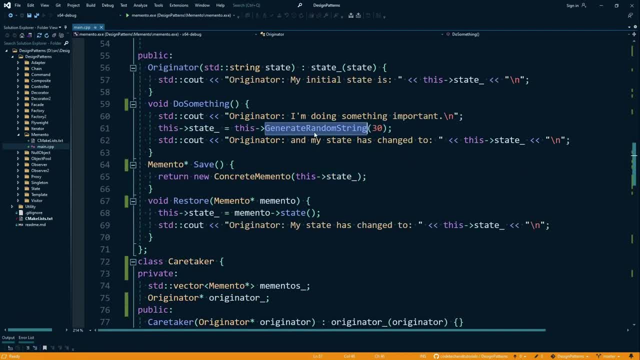 state. that's all they do really here with this generate random string, which is kind of cool. now they've got a save function and then the save- very important to know what happens here. it returns a pointer to a memento. so what's a memento? uh well, it's this thing. it's this thing. 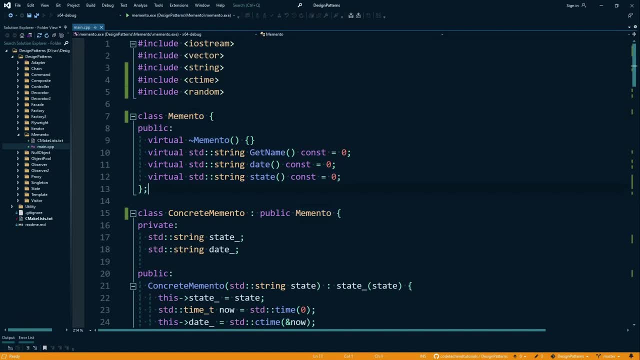 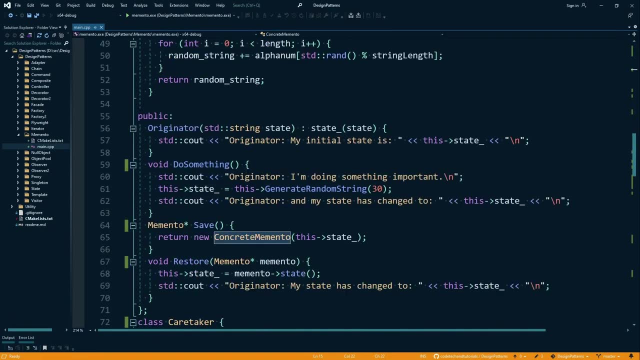 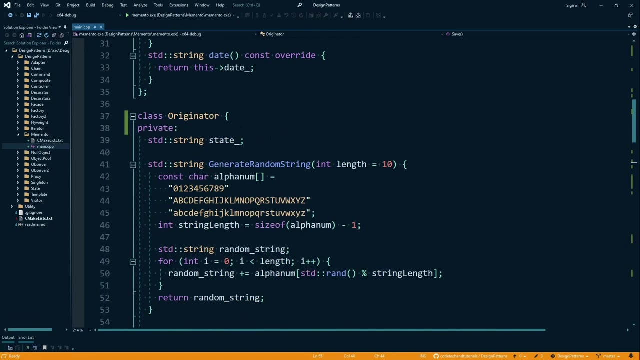 since it's a pointer. it's got to be a pointer because you can instantiate this base one. it's interface only, but when it's a pointer you can put anything that inherits it in that spot. so we're creating a new concrete memento and its state is whatever. 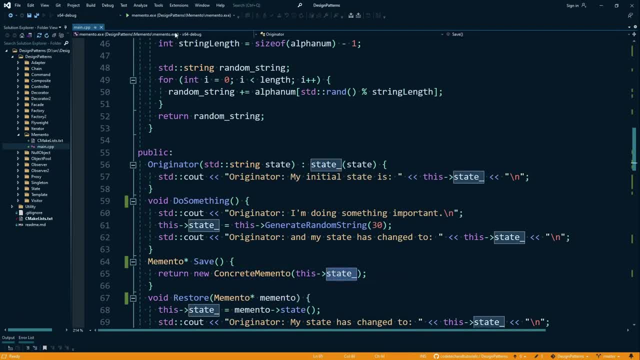 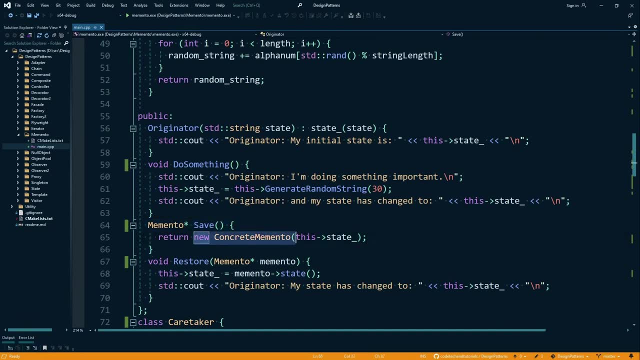 the state of the originator is right now. so there we go. that's essentially a backup of the state, and it's going to be returned now. note that it's not saved within this class. so where does this data go? it creates the data, it returns a pointer to it, but it doesn't save any reference itself. 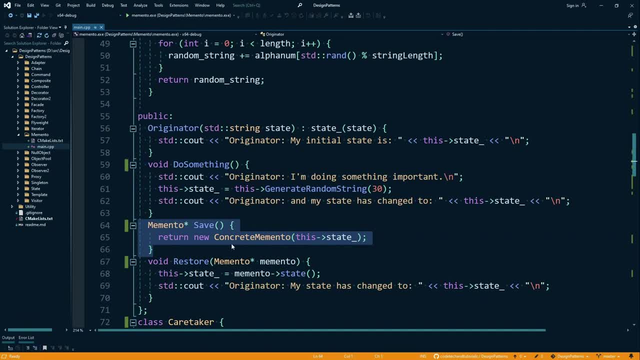 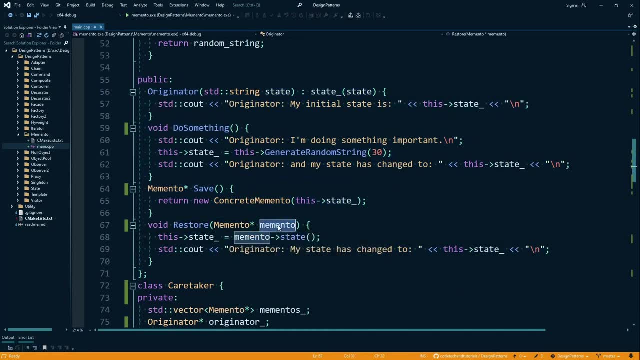 to it. so it doesn't really. this class doesn't know what to do with it essentially. and now we've got a restore method. note that these are public so anyone can call these. a restore method. takes a pointer to a memento- same case. it's got to be a pointer to memento so you can pass in. 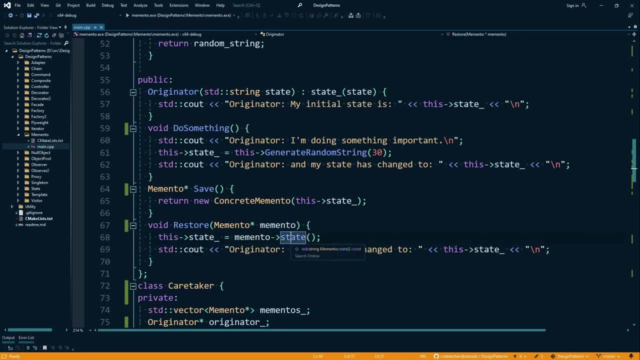 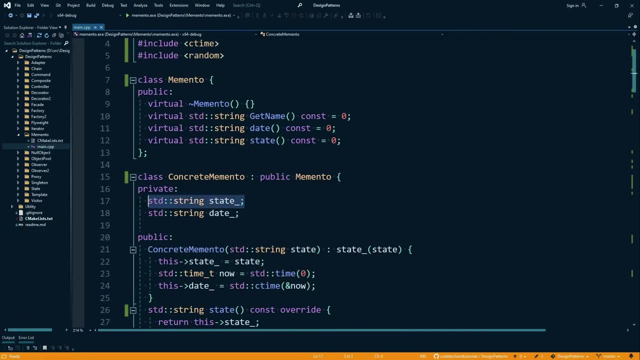 any kind and then you just set it to its state and you see how they get state here through this interface function. they don't have access to this here, this private data in the concrete memento. they don't have access to that, so they have to use. 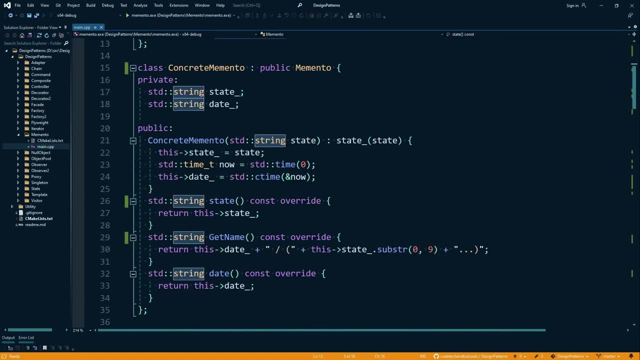 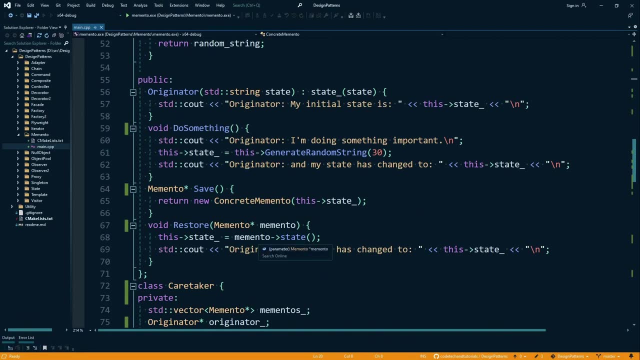 this public function that gets the state, and that was implemented right here in the memento, makes sense. so still, we're doing things properly with data. here is the point, and that just all that does is restore its state to whatever, whatever you pass in there. so you pass the memento, and so 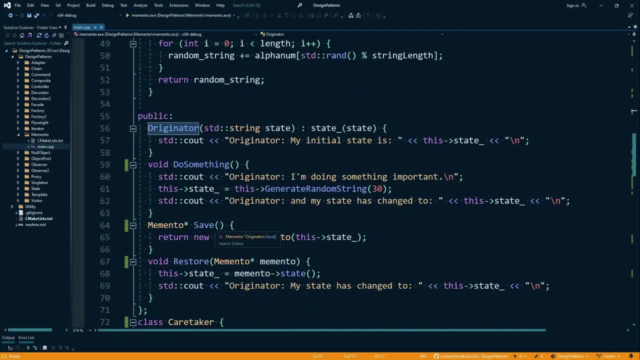 since clearly this class, you know, this originator class, you can. you can publicly press, save and restore, but you don't actually have any access to this internal data. there's no get state. uh, this automatically does it internally. you get this memento access, but with memento you don't. 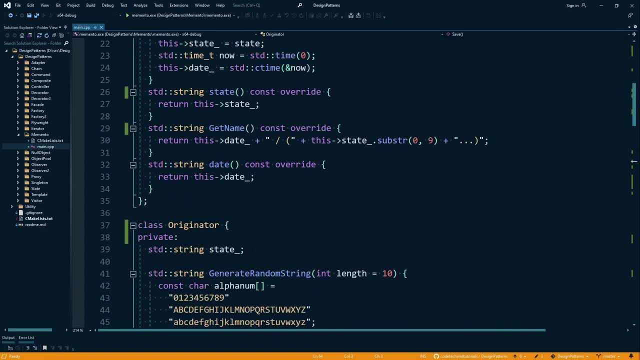 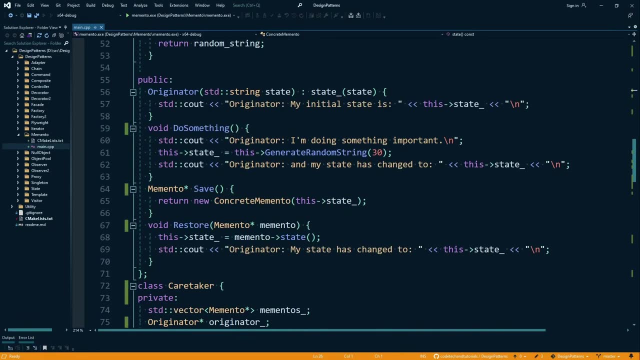 have. well, you have a, uh, you have a copy of the state, essentially. so, even if you get the state via this method, it's still just a copy, so you're not able to mess with the original data, all right, but to interact with these and interface with these and make them work together. we lastly need 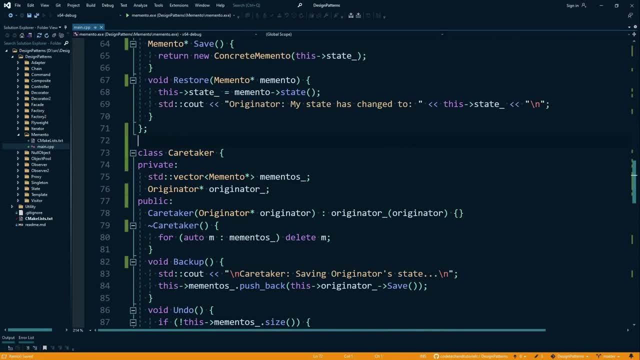 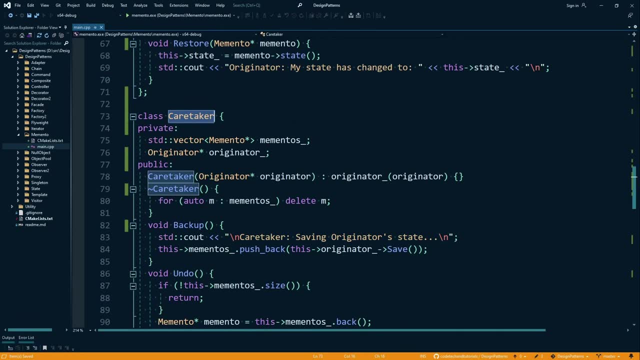 a caretaker. this is kind of the uh, this would be like the, the inner logic of your program. that kind of brings things together: the caretaker, mediator, whatever you want to call it. they call it caretaker in this example. so what does this have? well, it's got your stack of undo's, which is just 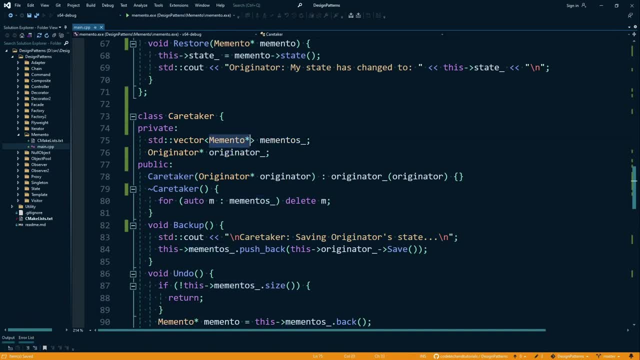 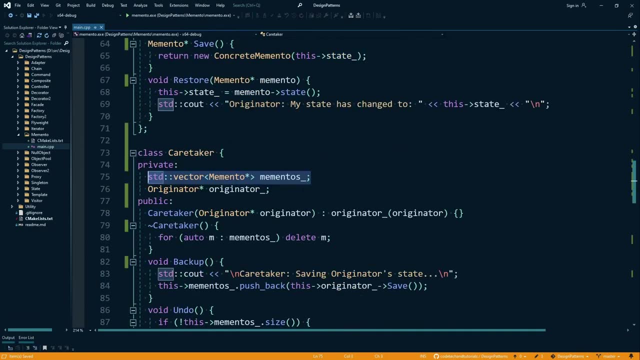 a pointer to all these mementos. we've got a whole vector of them so we can fill that up as needed. anytime we hit save, we can just add it. anytime we hit restore, we can just grab the last one and and hit restore. essentially is what we're going to do, and we've got also a pointer to the 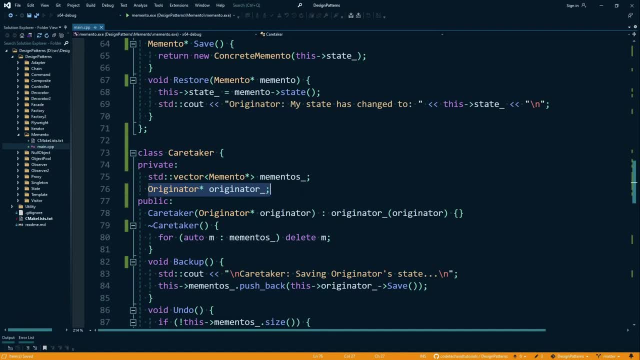 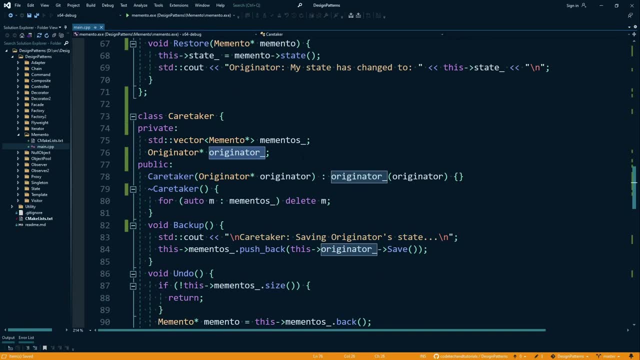 originator. pointer to the originator. somewhat interesting here. it depends how you're going to do it. if you're a true mediator, you probably keep the actual copy and manage the memory. it looks like here, though, they're not managing the memory to originator, they're assuming you. 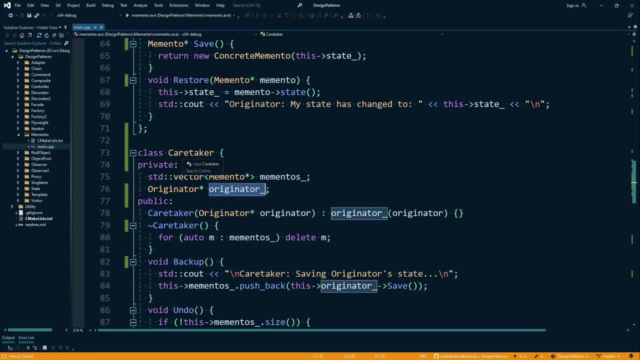 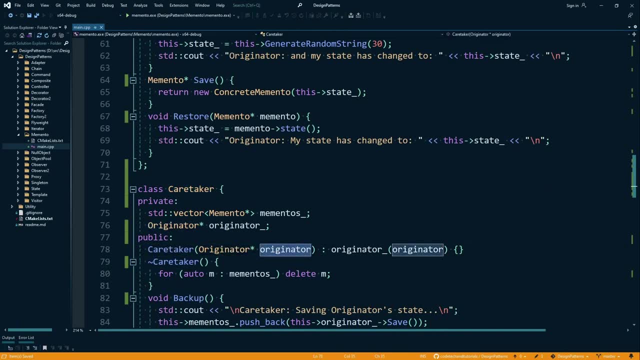 instantiated originator somewhere else and then later you instantiated this caretaker and when you created this caretaker you already have the originator. you just pass it a pointer. it saves its little internal reference. so this is more like a new originator reference. i would usually call these just because it's not managing the memory. 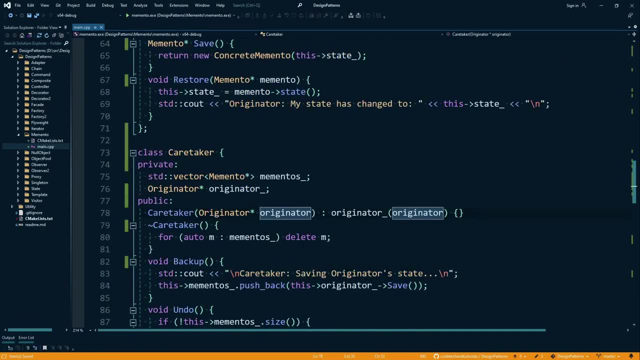 here. it's just taking someone else's instantiation, and we know that because we don't see anywhere in here where it says new originator. okay, yeah, because if not, we would say: you know, if we could store our own version of originator somewhere in here, you would see a new somewhere. 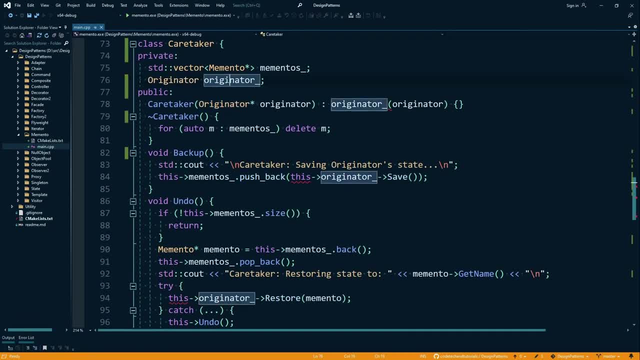 in here. you would see a delete, or you would just see this directly on in the memory, like so in the pointer that's already instantiated. all right, but since we don't have a pointer to the originator, that's not a good thing. just stop, and you can just keep going with what you're doing. so i'm going to. 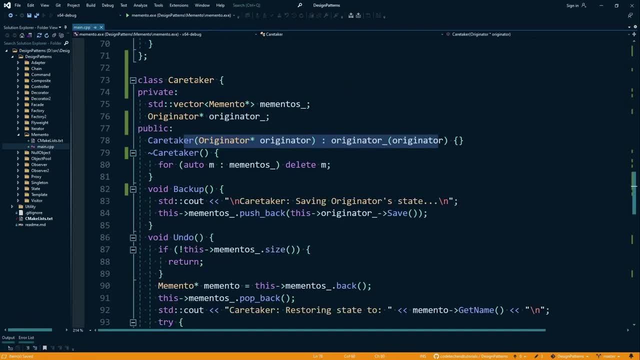 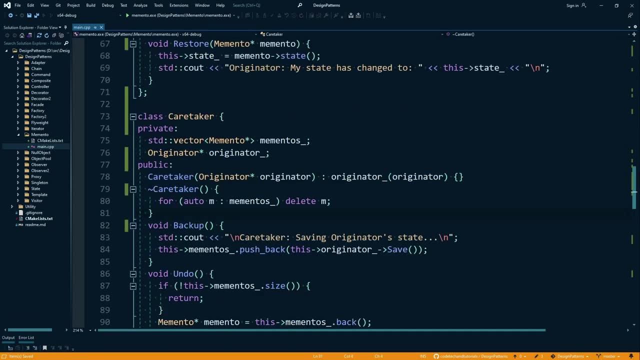 don't? we can see that we want someone else's originator to work on essentially, so this is gonna work on that, and you can see here. well, they do delete the mementos at the end. that's good, because you know these mementos are public, or? 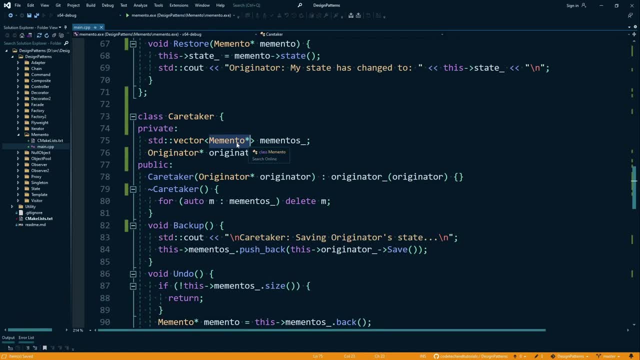 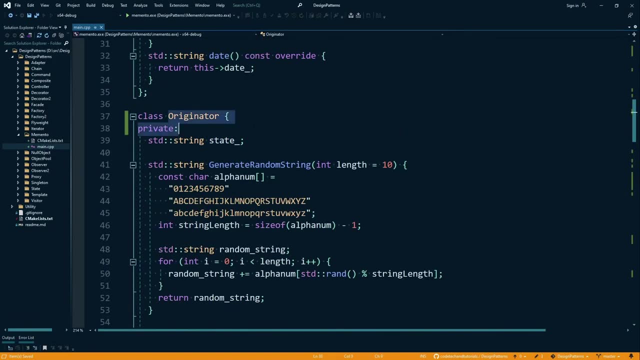 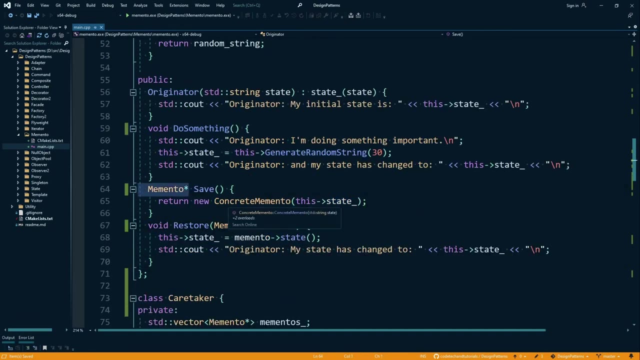 not public. sorry, they're private. these mementos are pointers, it's the word I meant to say. so we do need to call delete on them at some point and we already went through the entire originator and we know that it doesn't handle memory anywhere here and it is creating stuff when you hit save it. 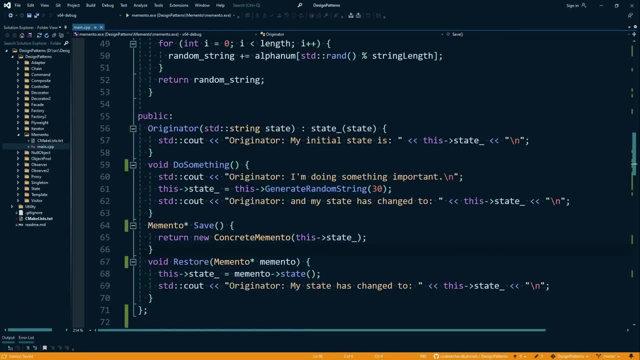 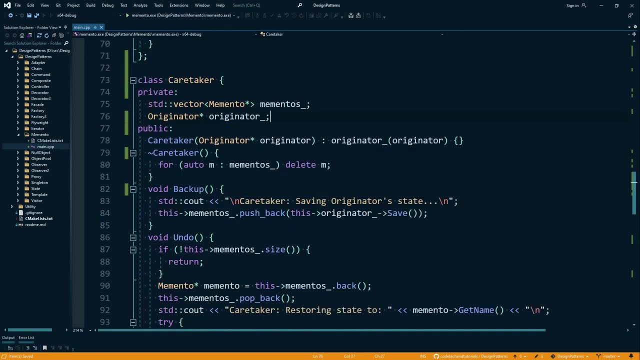 creates something but there's nowhere in here, or it deletes whatever it's making there, and that's where the caretaker comes in. it's gonna do that. we'll see that here shortly. alright, so we got a backup. now this is essentially the save button. so from the caretaker looks like you've got to press backup, and when that 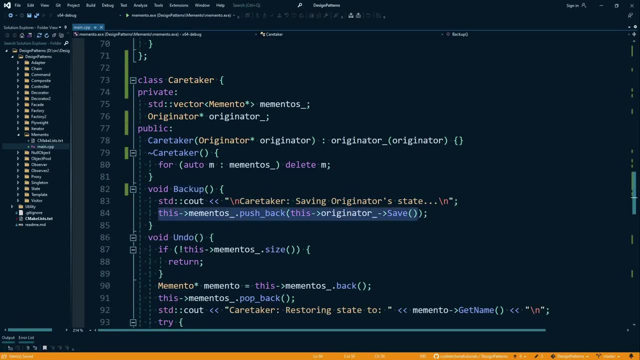 happens, it just pushes back a new save. now this is sort of interesting here and this is where I got a little, I don't know- queasy looking at the code and I'm gonna go ahead and hit save, and I'm gonna go ahead and hit save and 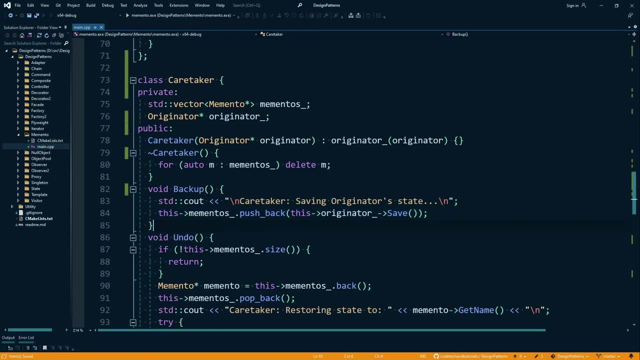 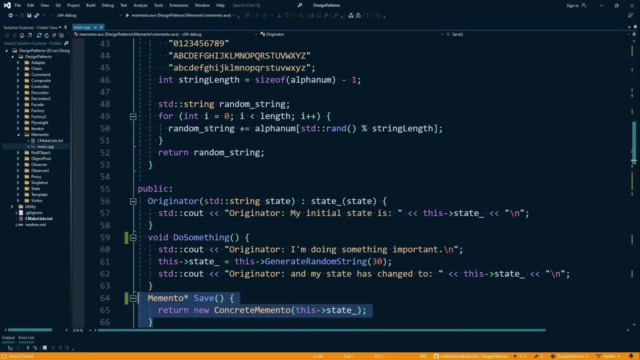 the code. I guess, because I was like wait a second- you're using the mementos method- backup- to call save, but the problem here is you have save public on the originator so any client could call save and what's good. what's it gonna do? 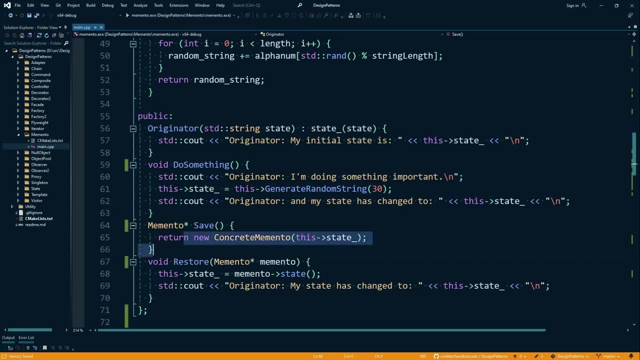 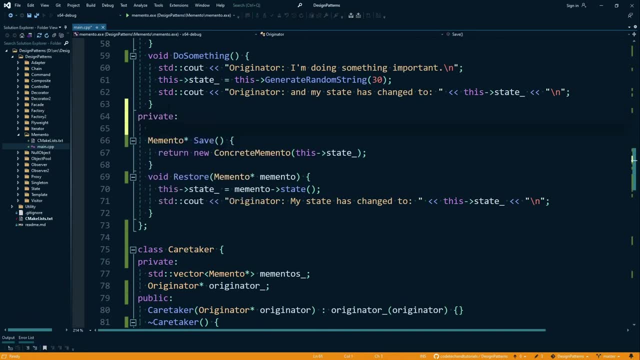 they're just gonna, they're gonna lose the memory. probably it's gonna memory leak basically. so there's kind of a bit of a failure there. like maybe what I would probably do is make this private or protected- no, yeah, private- and then make like a friend class caretaker, and that way only this caretaker class could ever call save and restore. 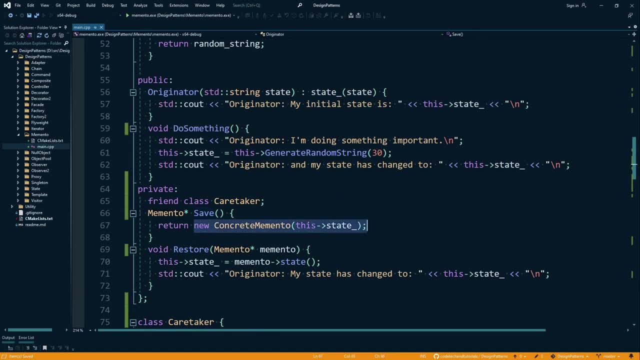 and that way the client can't just like create a bunch of mementos and like do who knows what with them, but probably not delete them and cause a big memory leak. so this way- oh this is pretty specific to C++, this whole friend class thing- there might be a better way, but I would recommend doing that. 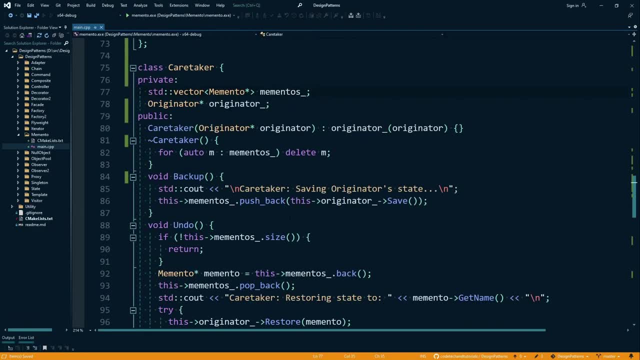 so there's one little edit we're going to make right off the bat just to kind of make it a little safer. um, so yeah, backup, basically just call save, as you can see, and it puts it in this stack of vectors. so we're keeping track of it and we know we're going to delete a later set. that's looking not. 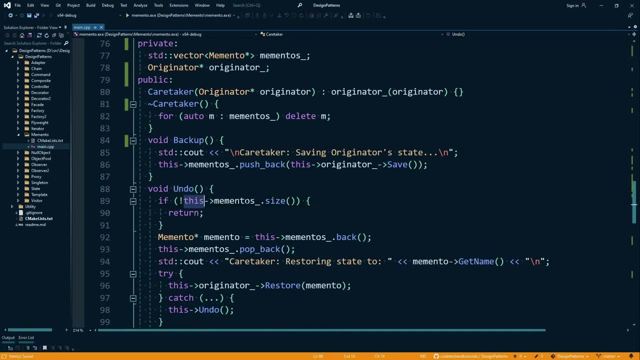 too bad. it's looking pretty good. we got an undo button and the undo button is going to well. first thing it's going to say: let's make sure the memento Size is greater than zero. basically, this is just a weird way of displaying that logic. so it's just greater than zero. 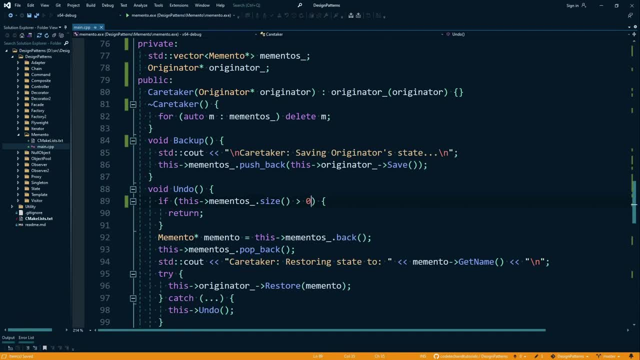 basically is what it's saying there, but with the not you know, a zero is going to be false, so they not false, which means it has something. however you want to write, it's fine. i like this, just because it's a little easier for my brain to unwrap if i'm skimming through the code when 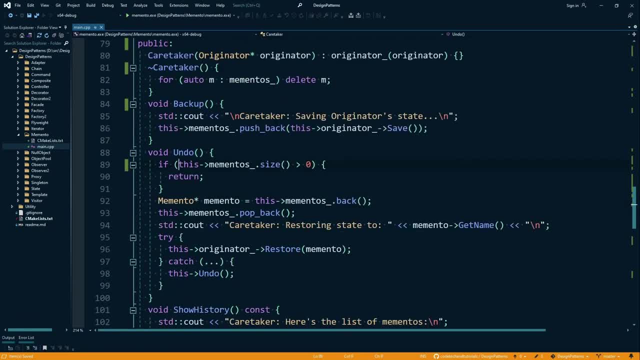 you have to think about. not false, okay, but it's a size, so when it's not zero, yeah, it's just. you know little extra logic steps. but anyway, let's move on. so here you can see, with this undo. first of all, they grab a pointer to the back memento. they just copy the pointer, not the data. they 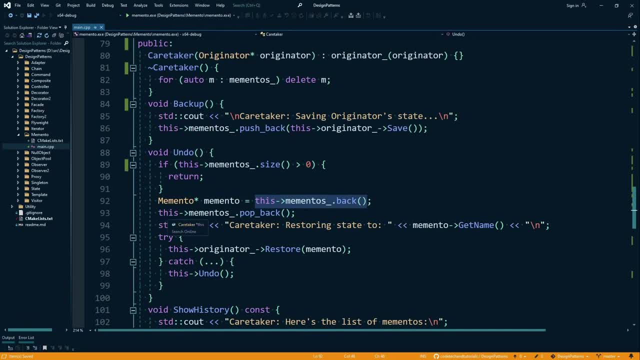 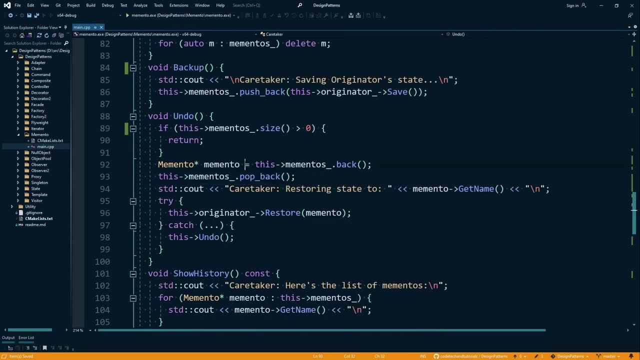 just take the very last one that's dot back there on that vector and then they pop it off of there. they destroy the back one. well, they don't destroy it, they release the pointer. that's okay, because we have access to that pointer right here. it's the very final one. uh, there's no more stored on. 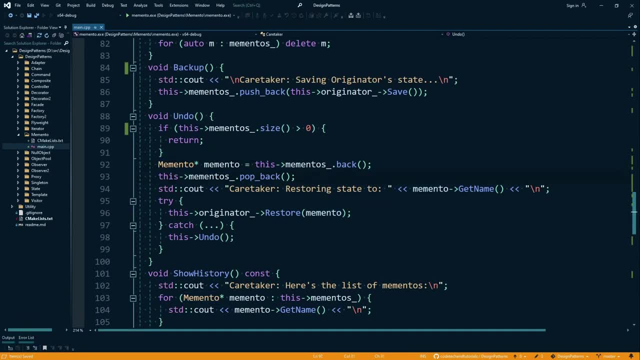 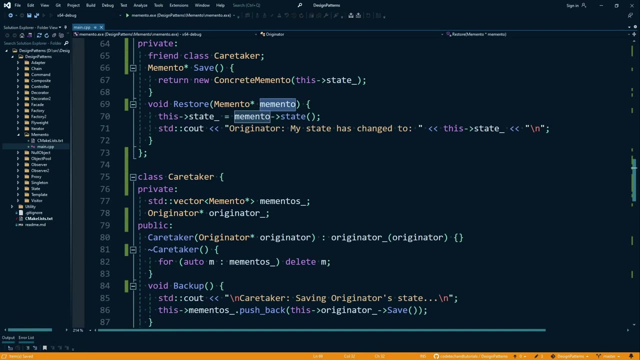 the vector. so you got to be careful about this kind of thing with pointers. um, so let's, let's keep checking this out, all right? uh, he tries to restore the memento. uh, so let's take a look at what happens here now. restore takes a pointer. it looks at the state. now this, could you know? if they don't, i guess if it's null. 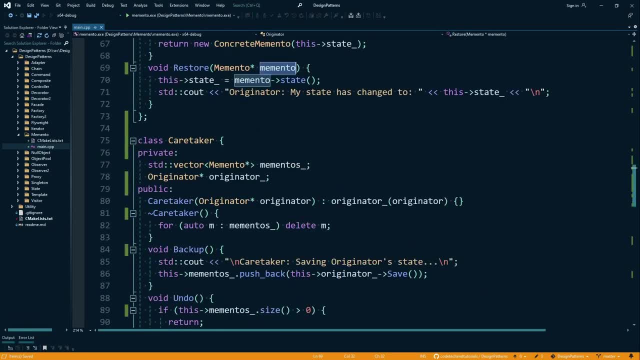 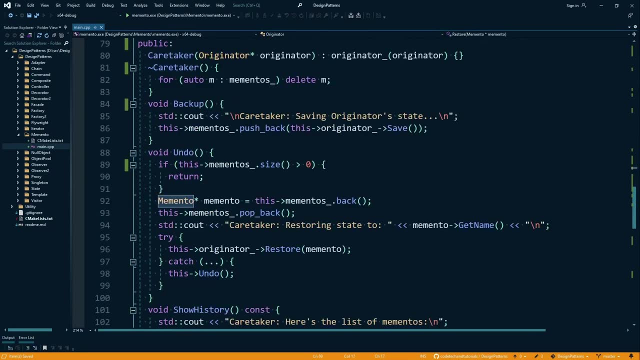 he would throw. so that's maybe why they have this catch here. but there's no throw within this function directly. it's probably just because it's a pointer. i'm not i forget, if try catch catches null pointer. i don't typically check that way personally. all right, so it tries to. 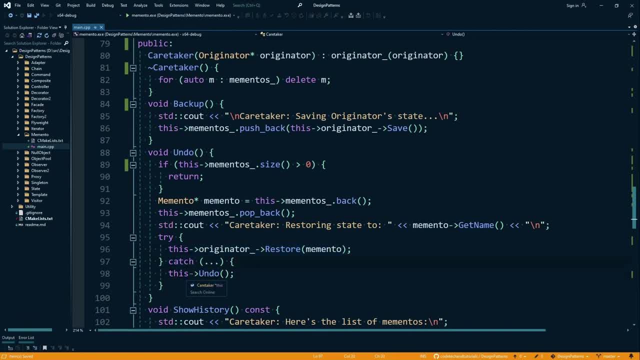 restore the memento, and if it fails, if it throws an arrow, they call undo, which basically calls this function again until it returns. so i guess what they're doing here is, if it fails to restore the last one, try the one before that, and so on and so forth, until it either gets one without throwing or the size is zero. 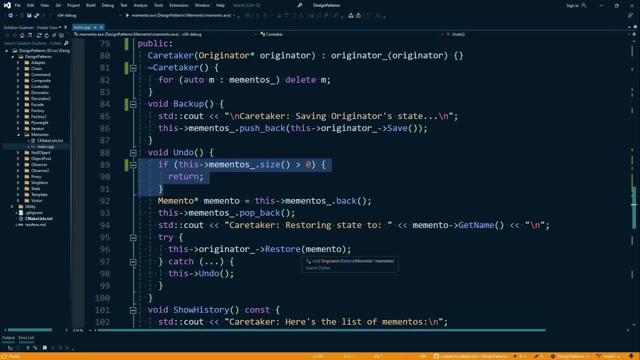 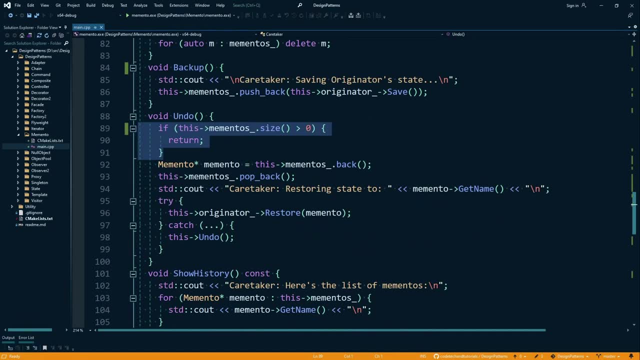 sort of a weird, weird way to process your undo, in my opinion, but it is what it is and they've tried to make it somewhat safe. however, they did leave a memory leak here, so that's pretty important to note. uh, let's think about this here. yeah, if i'm not mistaken, i might 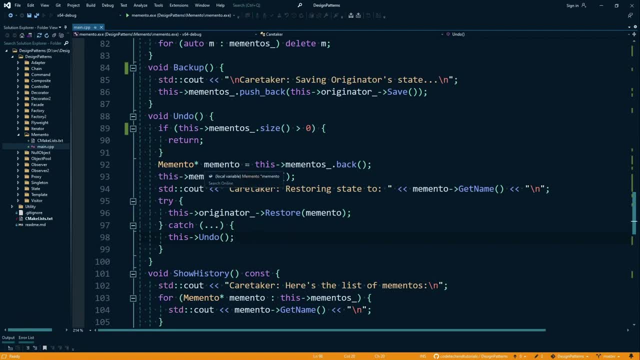 be mistaken. i'm trying to unwrap my head around this, but i think they left a memory leak because, well, okay, we've got a pointer to the memory that we just popped off the vector. this is the very final pointer to it right now, and then we try to pass it in to the originator. 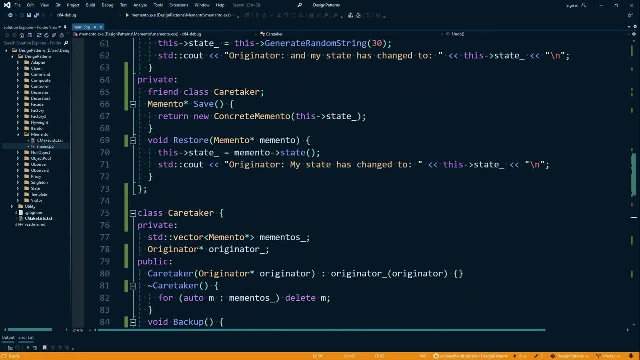 and the originator now has that pointer, so it it now has access to that last data state. and then what happens here is it makes a copy of the state inside the memento and it saves it to to this state. and now, when this restore goes out of scope, 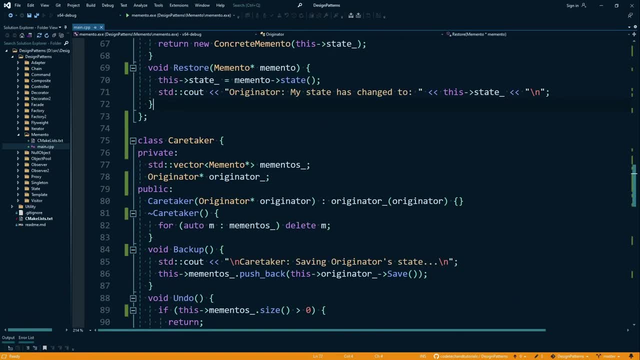 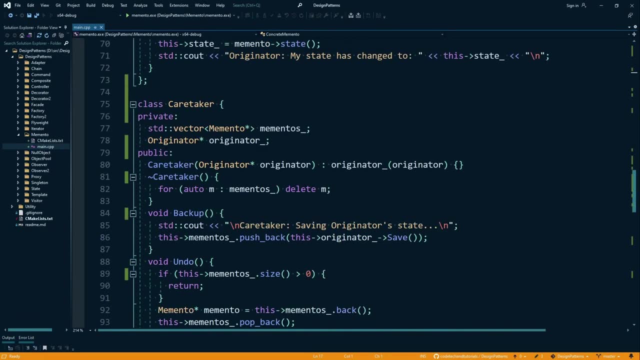 and this undo finishes that original data. uh, from this memento, which is going to be like a string, let's see here a string and a date that's going to still be on the stack. see what i mean. i don't know if that's going to make sense to you. if it does. 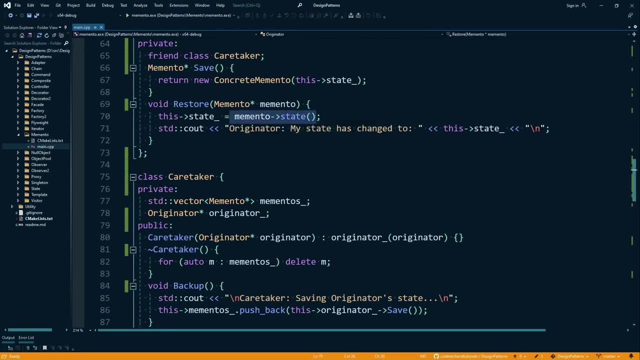 you understand pointers, but essentially, since they're making a copy here- 90, i'm pretty sure they're making a copy now- the compiler will probably optimize this away and it won't end up mattering. possibly, possibly, i don't know, it depends how it implements this. it should do a move. 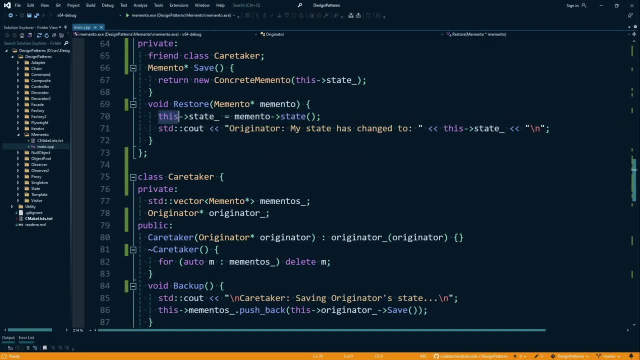 a move would be better here, because it would essentially say: you know, it would just, it would not do a copy and it would just say that this data is the data, basically. um, i think i'm saying that right anyway. so when these functions leave this pointer which has access to that state goes out of scope. there's no more references to that. 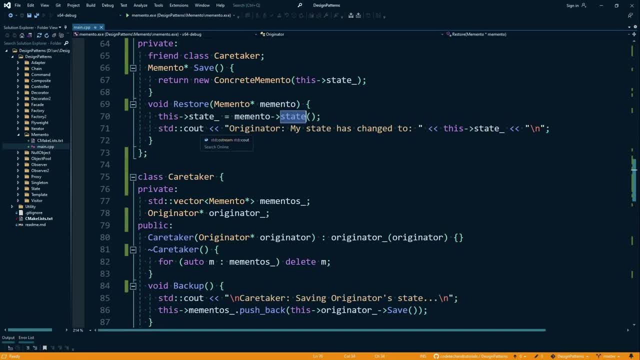 data that we copied into state, so we're going to have an extra copy of it. you know we're going to have it here. this dot state's going to have what we want. that'll be fine, but whatever was here is just no longer accessible. okay, i'm trying to make that clear because this is like the hardest part. 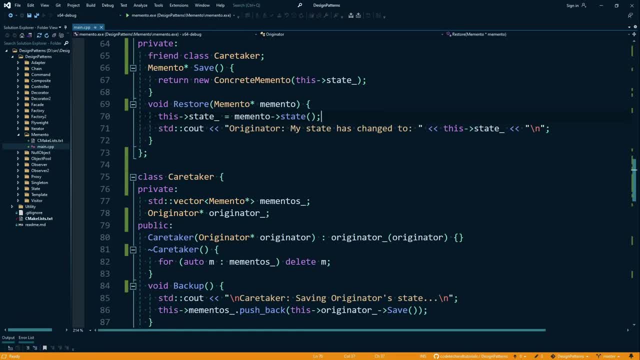 of c plus plus is understanding what's happening with data. in my opinion at least, and uh, that's kind of the point of c plus plus- is to be able to carefully manage it. you know you can't just so we're going to carefully talk about it occasionally because it matters a lot for 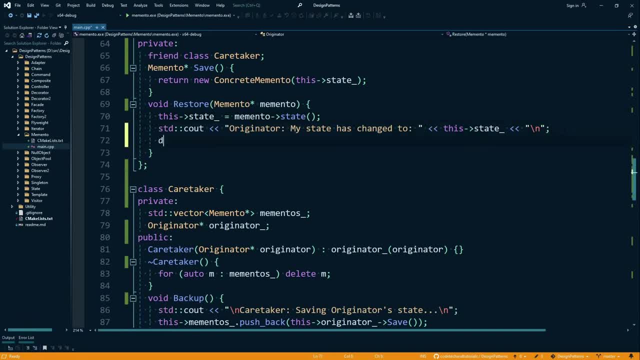 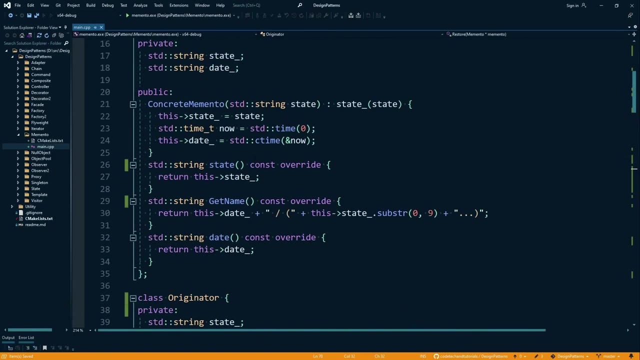 getting the fastest code you want, all right. so what we should do here is we should at the end here go delete memento, basically, and that will delete the state that has been restored, because we copied it anyway, since we did a deep copy there, and that's just the way this state function is going. 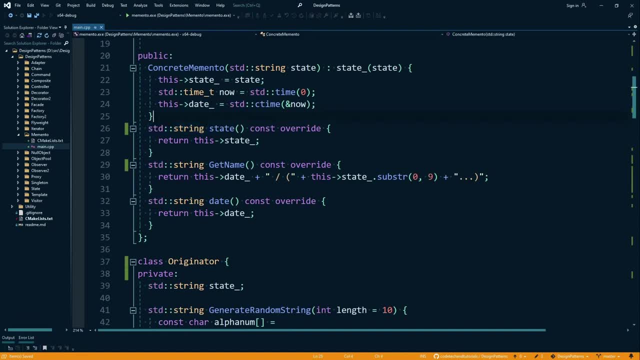 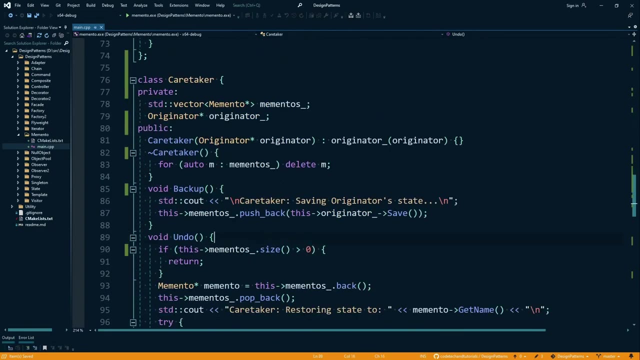 to work because it returns a copy of a string. now, if this was a reference like something like this: because it's returning access to the original data, not a copy of it, when you, when you do it like this, it returns a copy, so it's making a copy of that data. so that's why that would happen. 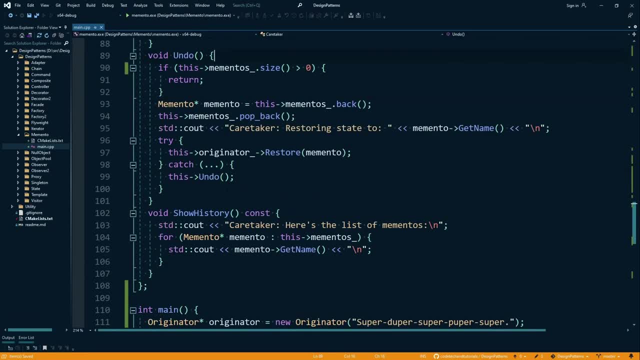 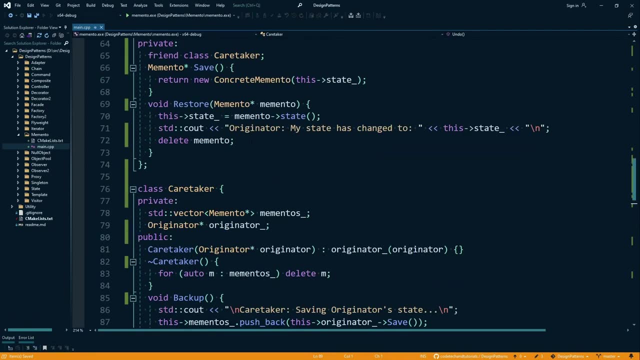 okay. well, we're kind of running out of time so i'm going to skim through the rest of this. i think we've gone through most of it undo function. you can see some of this needs a bit of work just to properly design it. you, whoever coded it up, probably rushed through it and didn't do a. 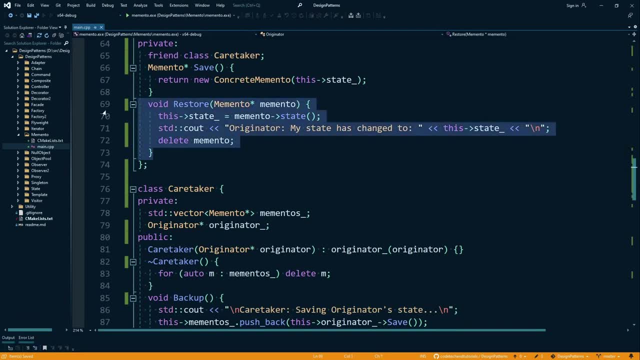 whole lot of debugging, but that's why you excited about this. um, so for the first time, i think we're things like this here would show up, should show up, as a memory leak. with any memory leak checker program you should get some warnings or errors there. so just because of the way, that's all. 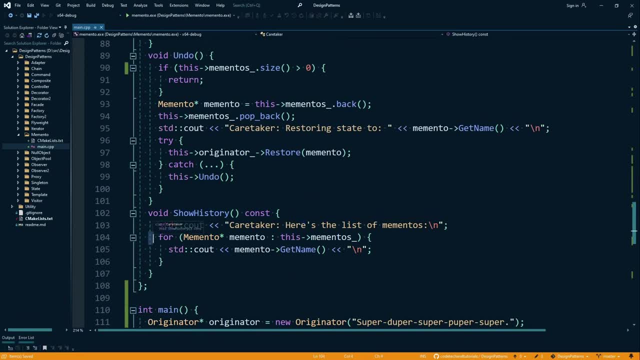 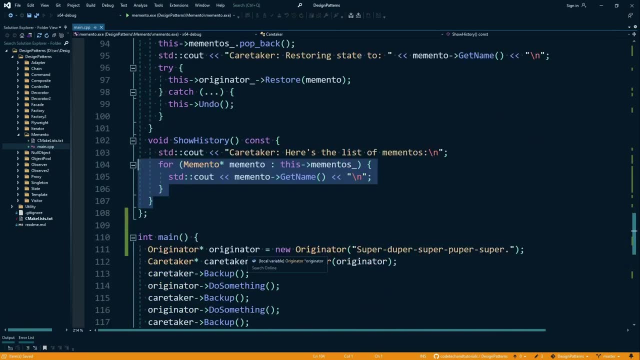 handled all right well. last thing, they have a show history essentially loops through all your mementos and shows you the names. nothing is super special, they're just looping through the mementos and showing you all their names. but that's a nice little functional little show history. and here we. 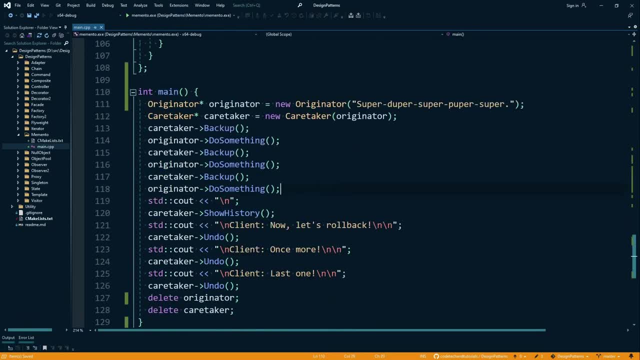 have the main, which is going to make our uh, whole example go. you see the instantiate, a originator here with some super duper, supper pupper, well, i don't know whatever. then they make a caretaker and you see, they pass it, this originator as we talked about earlier. then they call caretaker. 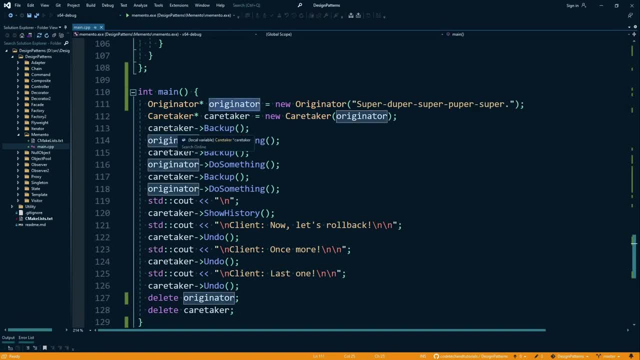 backup, which we know is just exactly the same as calling originator save, except originator save, uh, doesn't. you know nothing's nothing's store in the memento. you know nothing's store in the memento. you know nothing's store in the memento. no one's holding that pointer. that's why we got to have this caretaker intervene, but with our 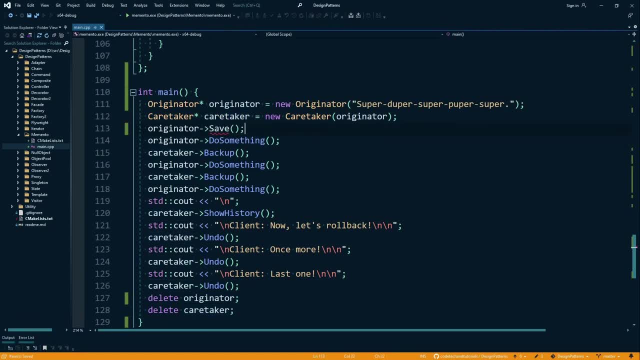 improvements. see, originator doesn't even let you call save, it's just going to say nope, unaccessible, inaccessible. that is better. that is better than the, than the way it was before because, as we discussed, that's going to cause problems. so that's the point of uh putting this. 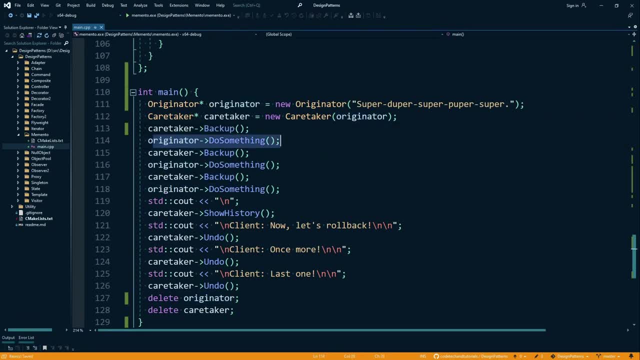 back up on the caretaker and then we see a do something which we know is just going to change the data and then back it up again. so you see, we're changing the data, save a state, change in data, save and state and so on. so we don't save after this last one. 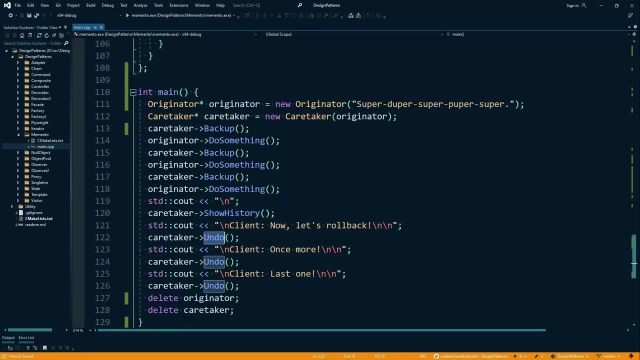 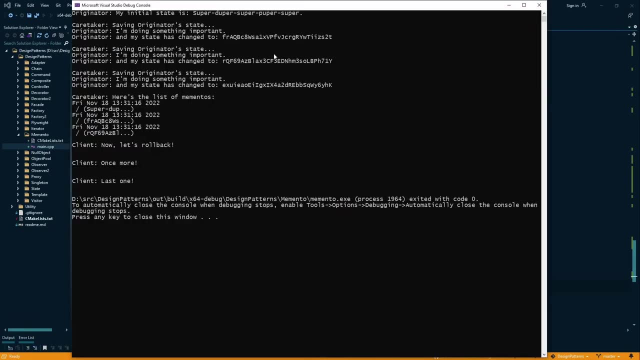 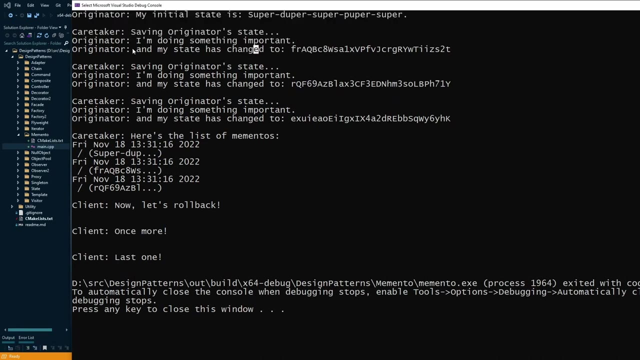 but then we just do a show history and then we do a couple undo's and then at the end we delete these. all right, so let's give it a run, see what happens. all right, cool, so let's walk through this zooming in again. there's the initial state um saving. originator state: doing something. state. 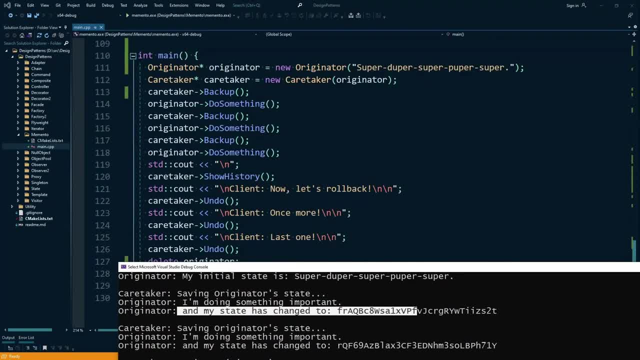 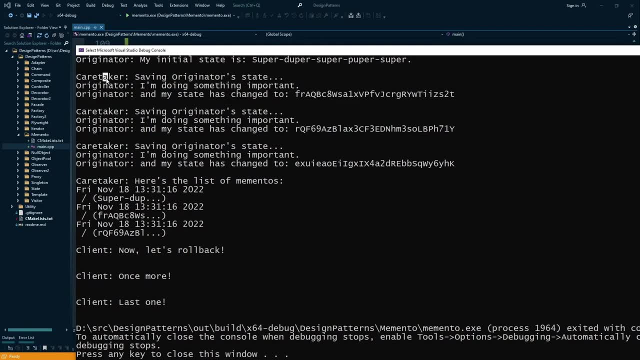 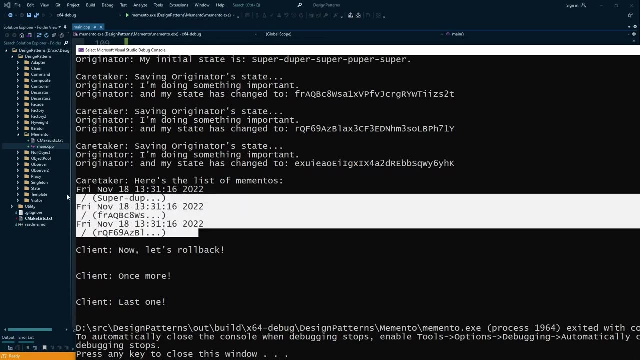 changed, doing something, state change, so they- they made it pretty verbose with all these couts- i think there's some couts in this- do something that shows this new state. yeah, they got originator and caretaker, so you can t see what. so you can see what class is calling it all right and then there's the list at the end. that's how. 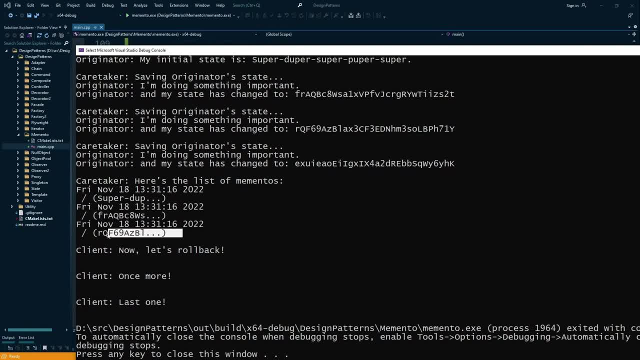 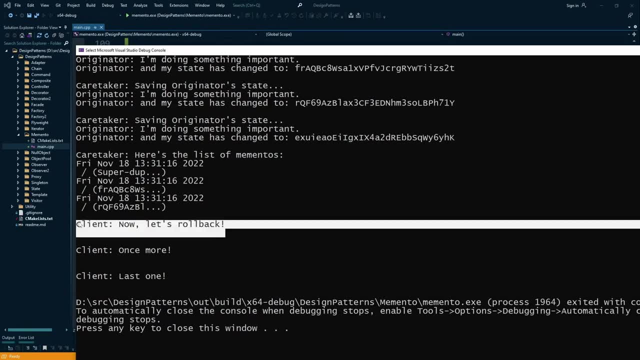 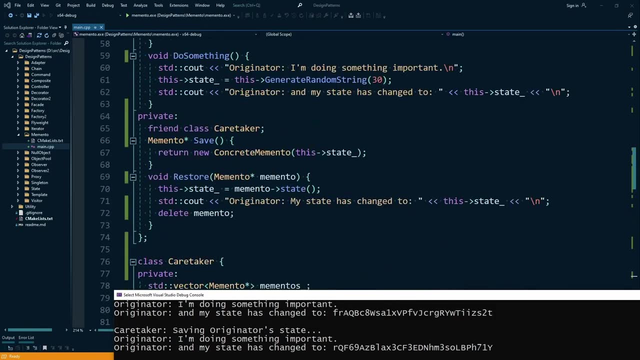 they displayed it. you can see the date comes in pretty clear and uh, there's the first nine or so letters and then, uh, we do some rollbacks- now rollbacks. we're not showing anything. after doing those, i guess we could uh show it state: how do we do we have a show state, uh, 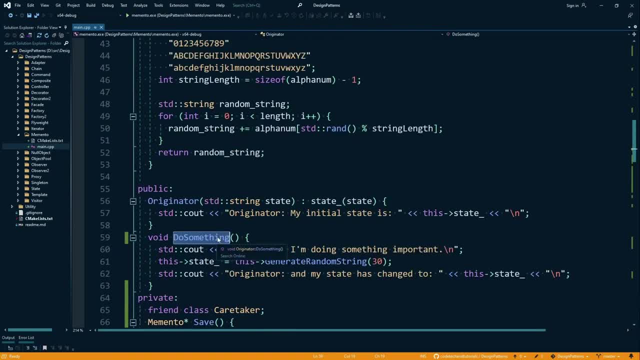 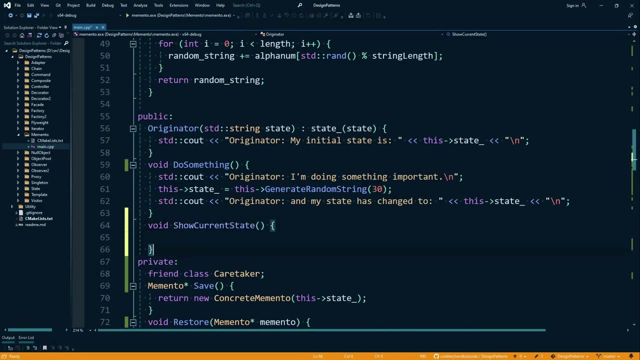 function here. no, all we have is a do something. oh, we could just make a quick show state, show current state and uh, yeah, let's just copy this down. yeah, that's, that's fine for now. we just want to be able to call this after each of these undo's. 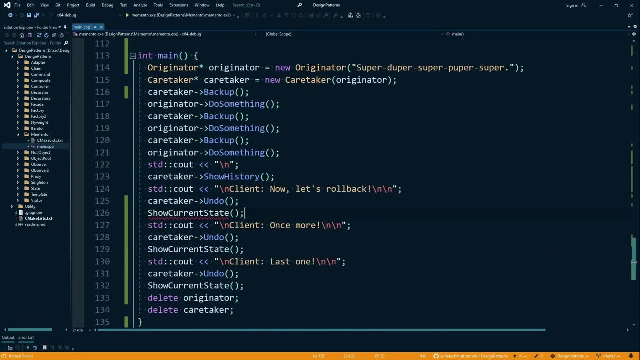 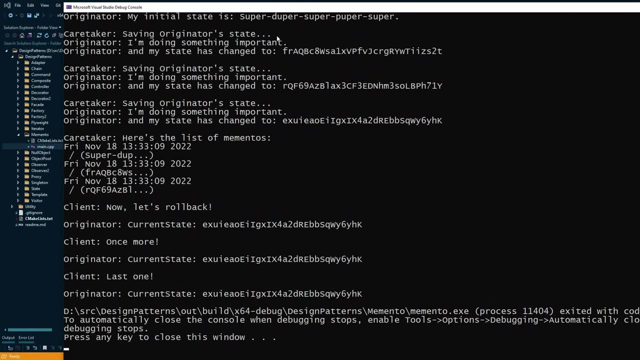 just to confirm that they are doing what they're supposed to do. of course we got to have the originator call that. all right, let's see what we get here. same code, rollback- says this current state is at rollback. again says this current state is this: it's currently not updating the state. 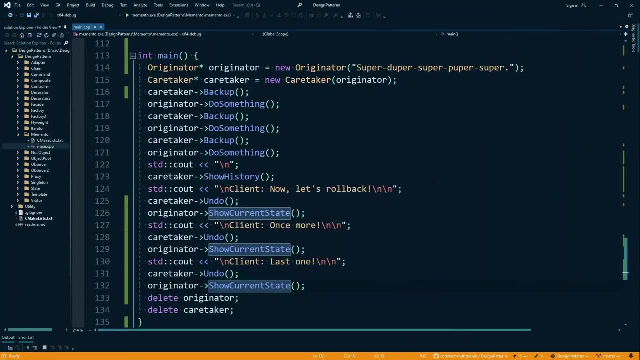 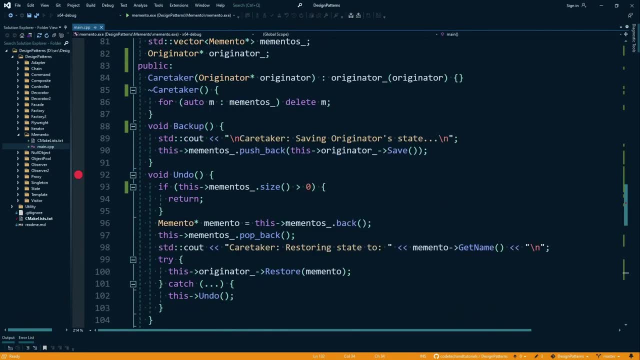 it's just staying as this last one. so, uh, what are we doing wrong here? all right, this is the part where i go full derp, or went full derp earlier, earlier when i was looking at this undo logic, so you can see i'm in a breakpoint here and i just took a look and it's just. 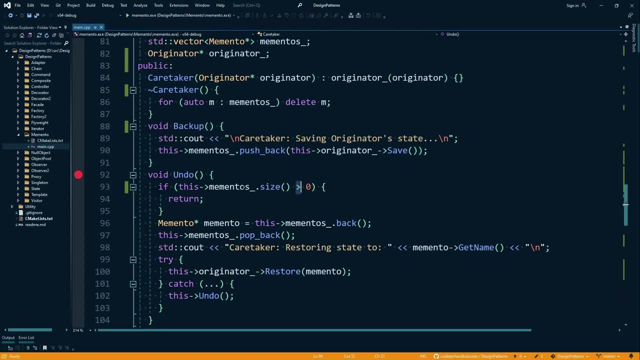 returning every time on this undo, so it's not actually doing the undoes. it's because of how i made this. if the size is greater than zero, returned. that's wrong. if the size is greater than zero, we can actually undo, so we don't want to return it's when the size is is zero. 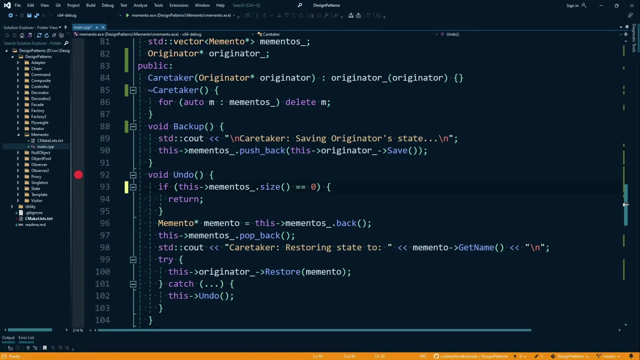 so we could say equals, equals. this would be a fine way to do this code. i like it better than the. i don't know. we can just leave it the default. i guess there was some merit to just having it like this right. if not size, it just reads so awkward to me. 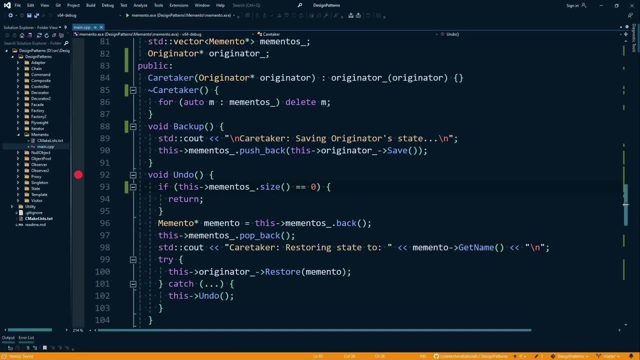 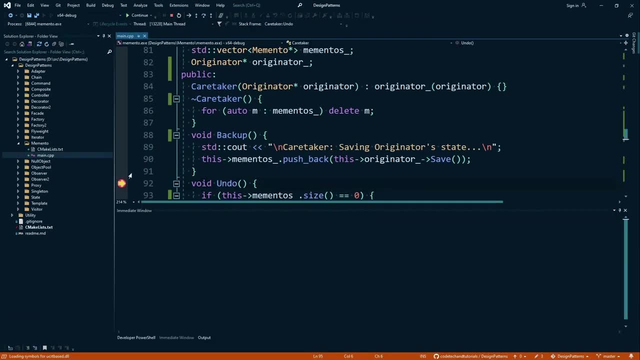 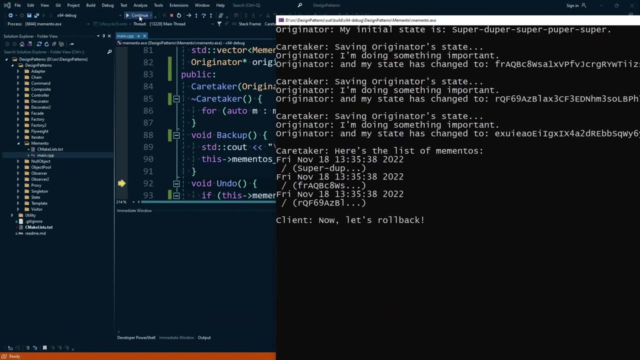 not size, i like equals zero better. so if size is equal to zero, return because there's nothing to undo. all right, let's go now. stopped at my breakpoint, but uh, there it is. we're starting to roll back. that's where i hit undo and i'm just going to hit: continue. we'll go through the rest. 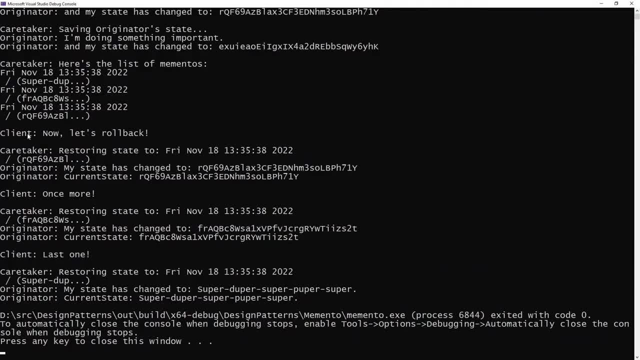 and take a look at the code. all right, looks like it's rolling back correctly. now we got a restore state there and, uh oh, we're accidentally set it up here, so we're going to go ahead and hit it twice now, because i put that current state function in there. i was overlooking the fact. 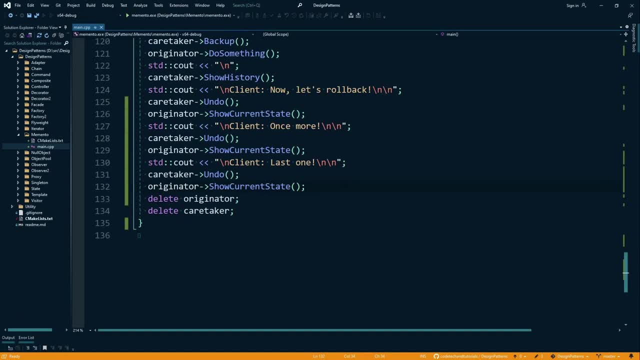 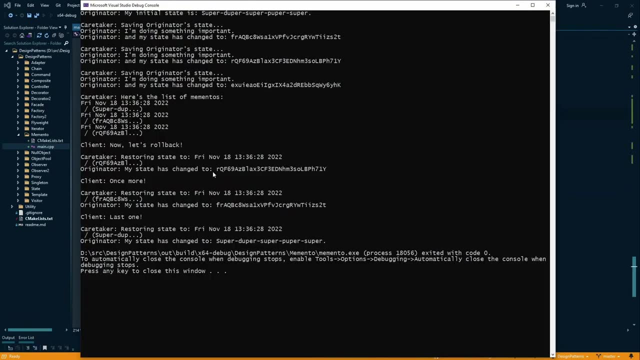 that they had it right here already, since it was skipping over it. but no matter, uh, we can just. uh, we can just delete this extra line. not too big of a deal, but this is what we wanted to begin with. okay, so now you can see it is actually rolling back correctly. current state is this here after: 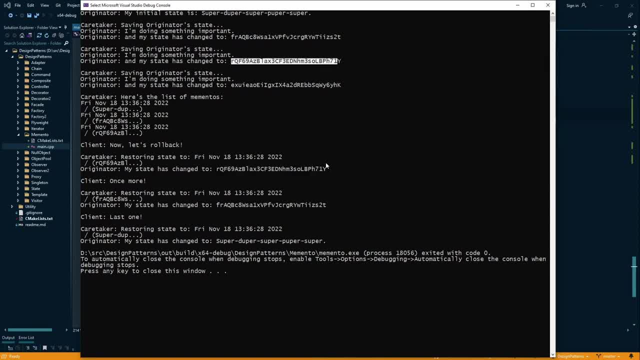 a rollback, it is now that previous state. after another rollback, it is now that previous state again, and after one more it goes back to its very original one. so we made four changes, we made four undoes, or three changes and three undoes. we're back to the original state. it is working as intended. so 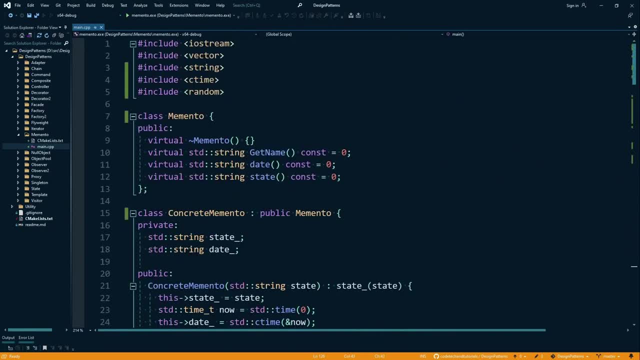 there is a pretty standard way of doing it. this is probably the best way to do it with this interface class. if you can't do interfaces, i'll talk about that briefly here. so essentially, if you can't do an interface, like if you just gotta get rid of this and get rid of this, things change a bit. 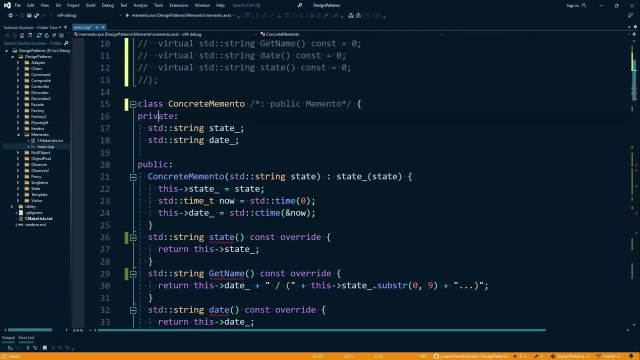 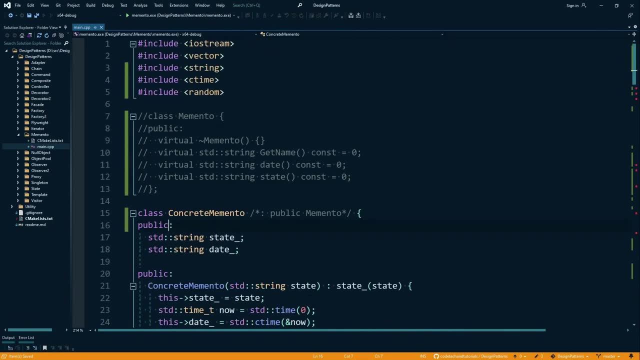 obviously you wouldn't need override here. well, basically, what you have to do is just is just make these public and let it have direct access. so if you can't use the interface for these type of functions, you just got to expose it, not a whole lot around that. for some languages it still. 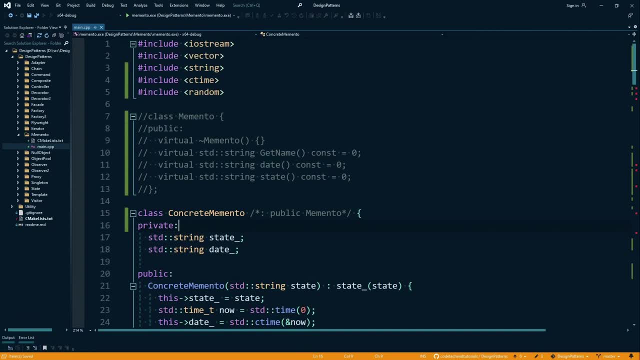 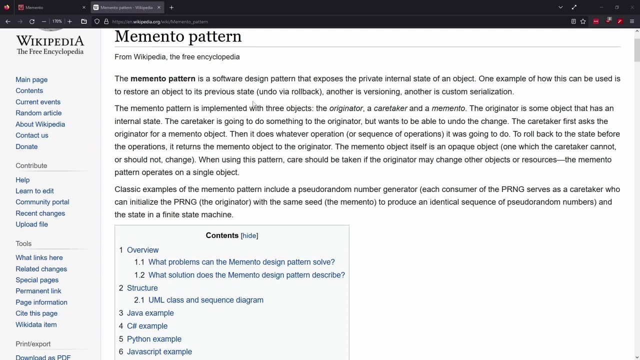 works. it's just a little bit more dangerous and people can misuse it easier, so you got to watch out for that. um, rather than talk about all these different methods, i'm going to leave you with the reference right in your face. so there we go. the wikipedia entry on this is pretty good. 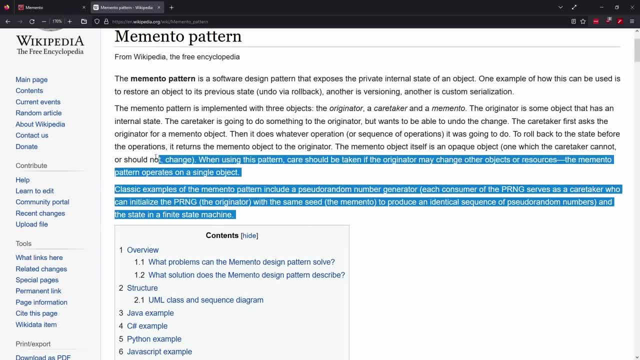 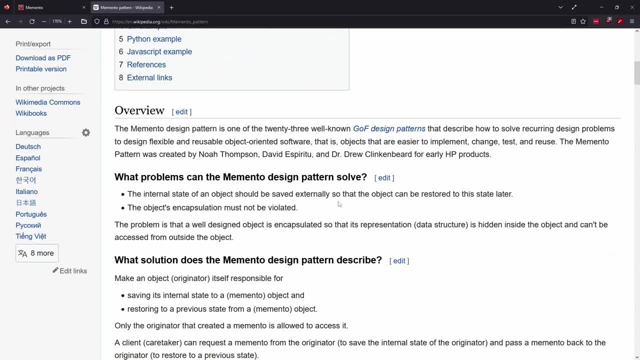 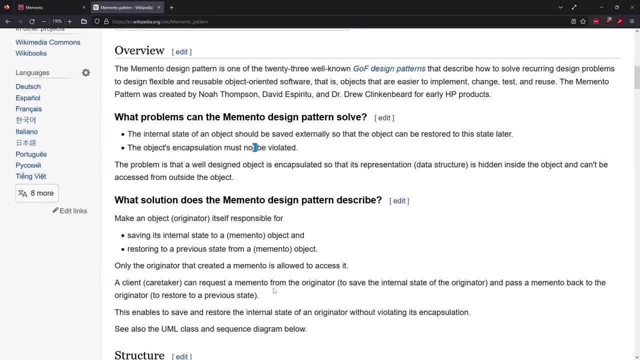 and covers a lot of stuff, including some classic ways it was implemented, such as for the pseudo random number generator, and it also talks a little bit about where it came from, who created it originally- not that kind of stuff which is kind of cool info. they also make some. 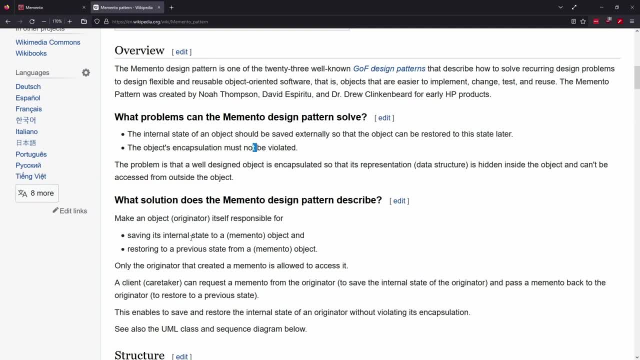 mentions of other ways of using it, but essentially it's what we went over. the originator is responsible for saving and restoring, but not necessarily for storing these backups. so they assume the client or a caretaker will be requesting these mementos via save and they can. 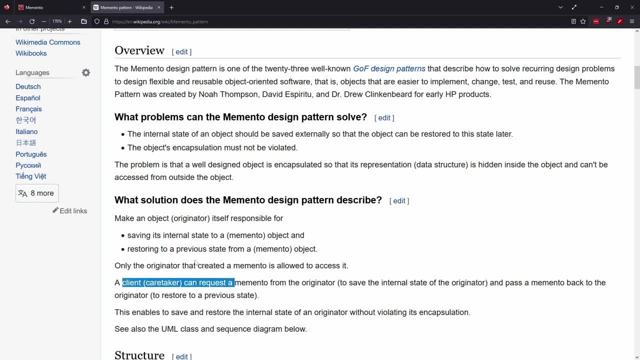 control when restore is called, to pop it back in there. so there's a little bit of variety of ways you can use kind of that caretaker or client, depending on how you're calling it, the save and restore. so you could- you could in theory- say hey, it's the client's responsibility. 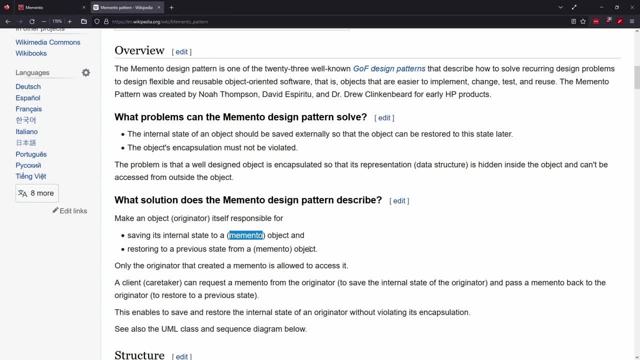 to manage these mementos of saving and restoring, like here's the type, here's what it's going to return and here's what you restore as. but sometimes i might not supply a caretaker, sometimes you might need to make your own vector of mementos or whatever. so there's. 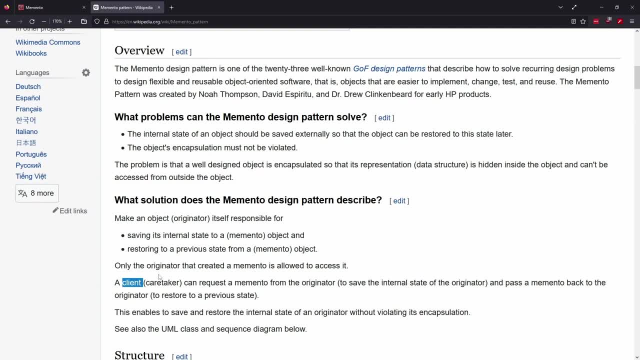 kind of one design difference there. in ways it can go, uh, the way we did and the way we uh edited the code and fixed a few things, is we assumed that there's always going to be a caretaker, because we actually uh shut off that's having the client save the client has. 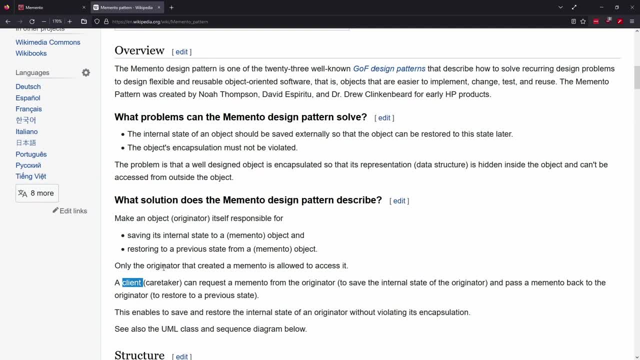 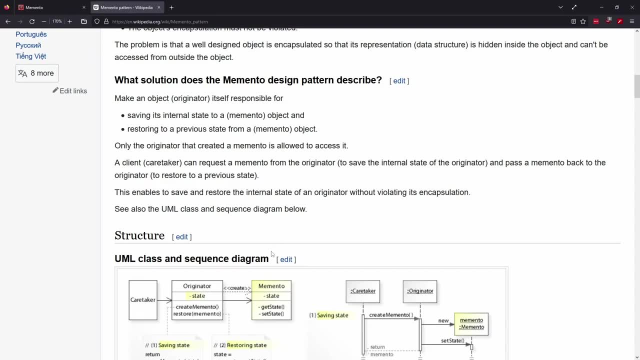 to use the the caretaker. they can't, they can't restore or they can't save and hold a copy of a memento. that's that's where we did that private thing and the whole friend class caretaker. so there's one little difference there and there's a lot here. they go into some more examples, but 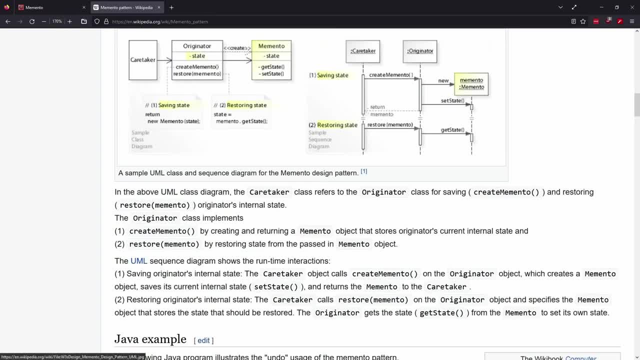 essentially it's the same stuff i've already said, but if you're having trouble getting a grasp on this, i would recommend just trying the examples yourself first, and then, you know, reread and rewatch if you need to. but all right, let's see what else we can find here for varieties. 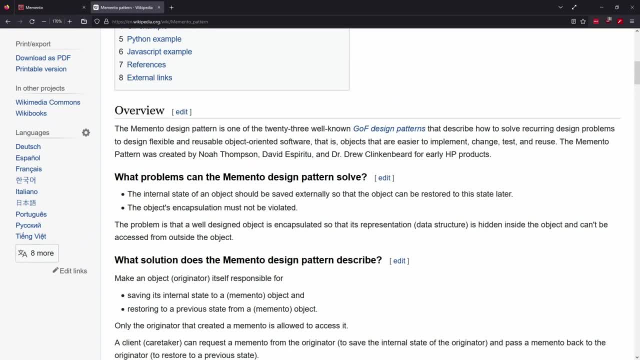 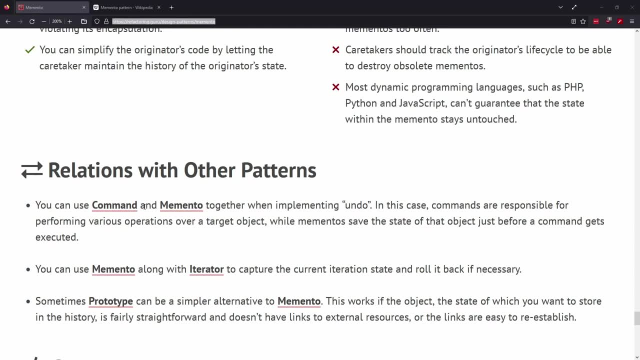 i'm trying to find the place where i originally read this stuff i'm talking about and i don't remember anymore, okay, well, i guess another thing where i was kind of calling the uh caretaker like a mediator. in this case they're sort of referring to it more as a command, just because of the way it. 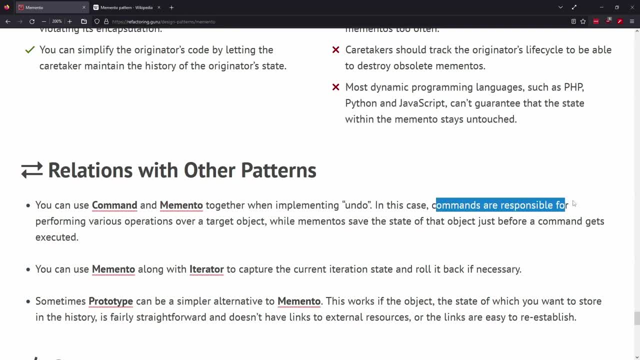 has uh commands, i guess. so yeah, they seem to be more saying: the caretaker is a command object, so i guess it passes in the memento. commands is what they're referring to. okay, no, i'm slightly mistaken here. so what they're saying with command here is: if you're using 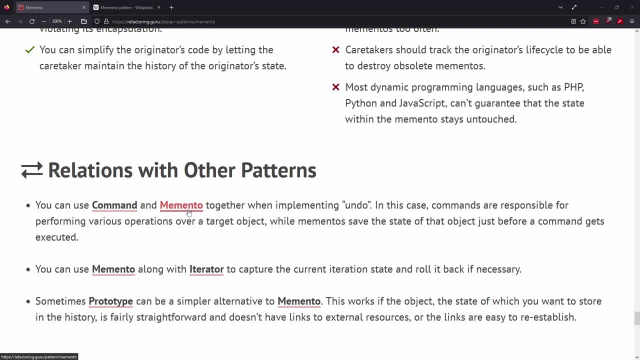 command, you obviously you optionally- have mementos in there, so it would save the state of the object just before the command gets executed, meaning that, you know, basically functions like an undo, because anytime, for example, if you're making a text editor, anytime you press a new key it's going. 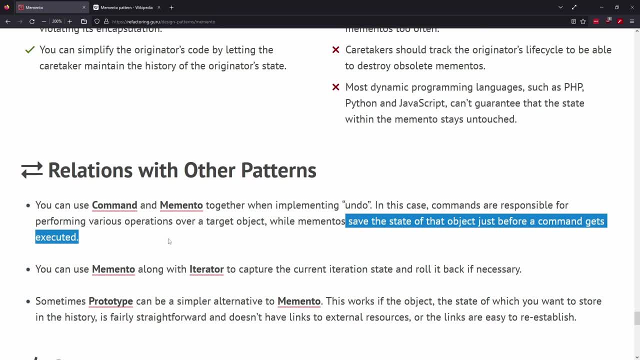 to save the state before putting that key change in there. that way if you hit undo, it just undo does it, so that makes a lot of sense. so sorry for the confusion there. it says you can use it with the iterator, which sure makes sense. if you're just sticking with the vector, most of that's already done for you. but 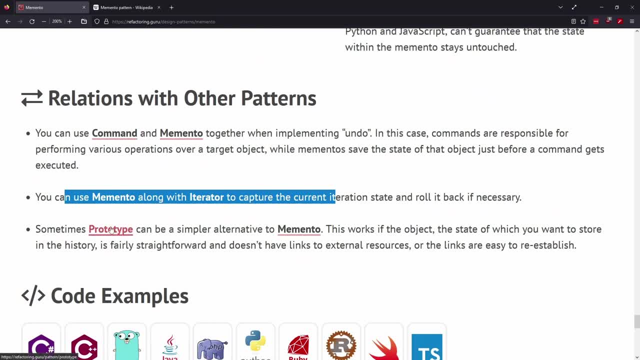 if you need to implement your own, doing some special stuff, that might be a really good experiment too. there's mention of the prototype being just a simpler alternative. now, if you remember prototype, it's basically where you're making a copy of something in a very specific way and then you just copy it. 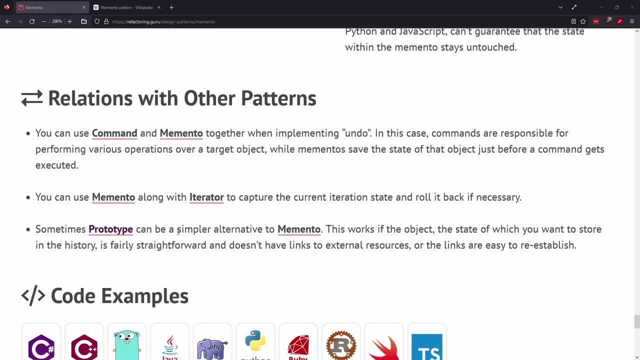 back. it's a lot like the memento, just a little bit more simple. really fairly straightforward. if it doesn't have links to external reference or links are easy to re-establish, it says, okay, so maybe check out prototype if you want to compare and contrast. but they are actually. 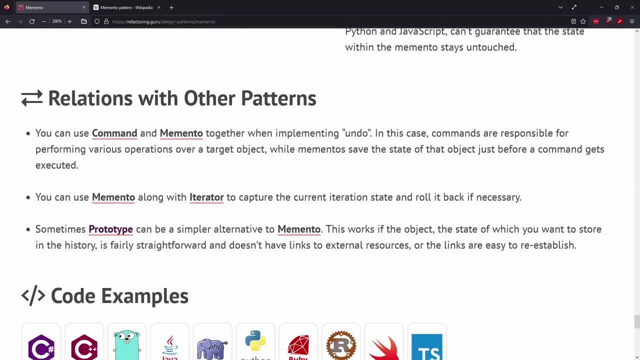 in a lot of ways. quite simple, they basically do the same thing as far as restoring state, because prototype is basically made to copy the same state, while memento is more about restoring states. but hey, if you are saving each current state as a prototype and to restore later, you. 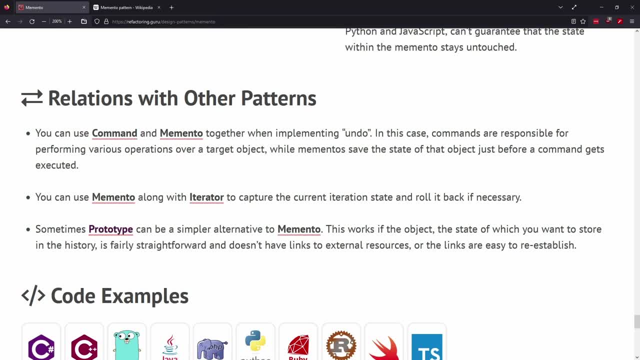 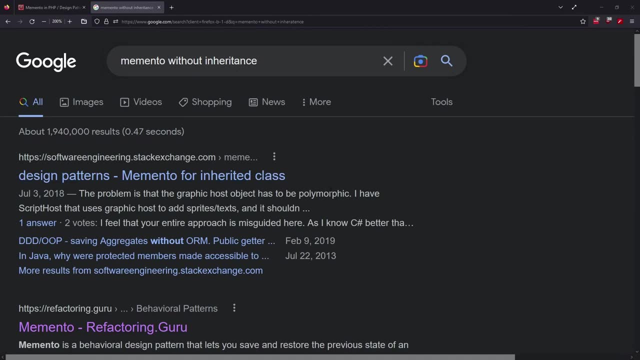 know there's a bit of mash up there, so i guess it depends how you implement it, what you call it in some cases, but memento kind of. i guess people are used to hearing that- for the whole undo process all right. and the other one was well, memento without inheritance. i tried to find the php example. 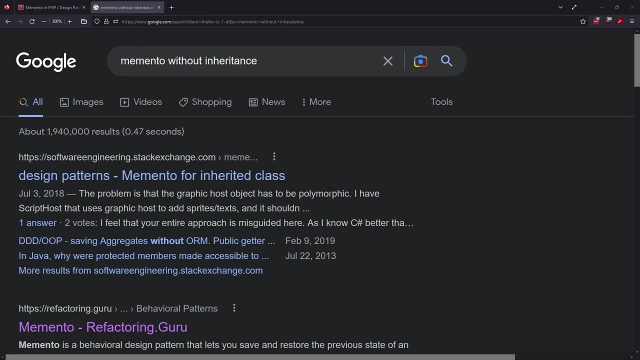 it looks like at least modern php does support some inheritance, so that works about the same. but the other way around is that you can. you can copy the star and paste it in the same way you want to, and if you want to, you can just copy the star and paste it in the same way you want to. 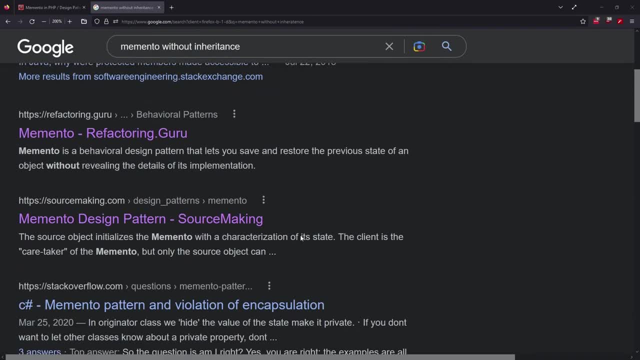 but the other way around is that you can just copy the star and paste it in the same way you want to of doing it is without inheritance, and that's having a little trouble finding examples on that. i read about it somewhere at one point, but i can't seem to find it again. you know it's one of those. 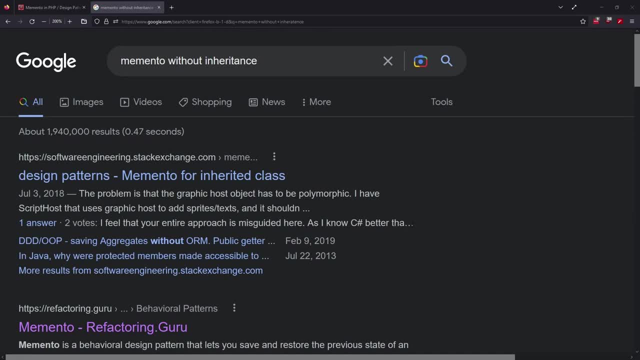 things, but essentially you just have to expose some things, uh, as public. usually those data members probably be more prototype-esque in this case and uh, yeah, i think that's all i got for this video. hope you enjoyed once again. don't forget to hit like uh, leave a comment, subscribe if you want. 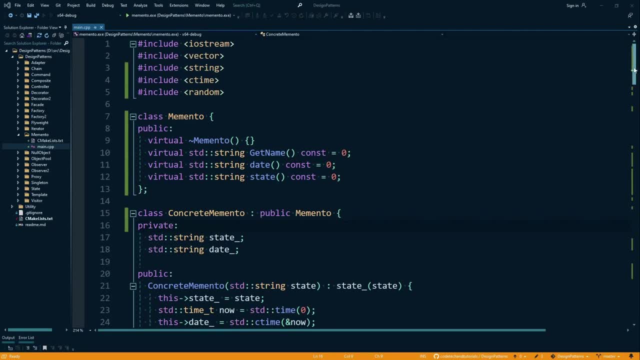 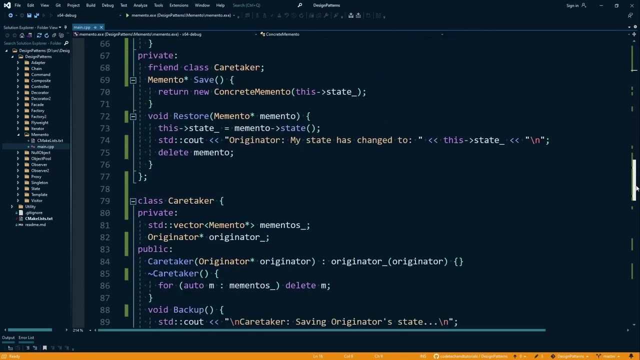 to see more stuff about c plus. plus, you can join the patreon if you want to get on discord and have some further conversations or ask me anything, especially after this video's been out a while. i might not be responding to comments much anymore, it's just the way it goes, but uh, yeah, this code.